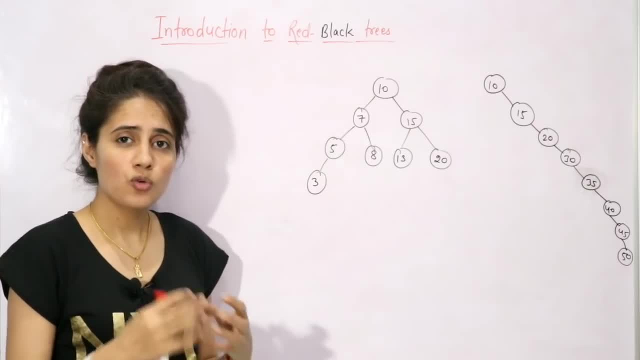 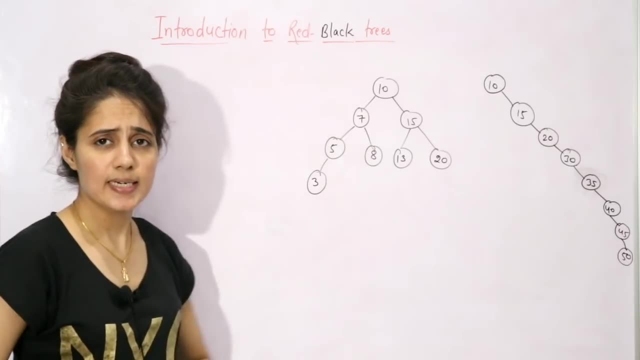 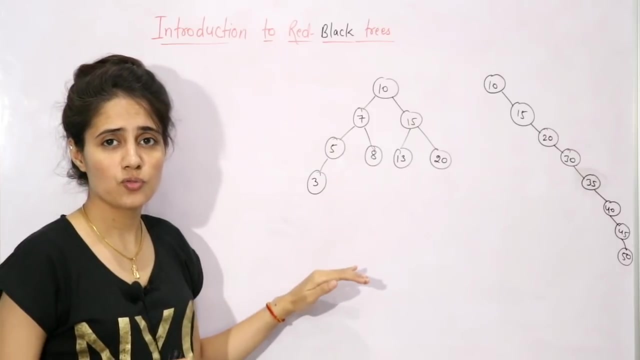 is what you can say, that frequent operations, what type of frequent operations you are going to perform on that data right? See, in tree data structures it is red black tree is basically a binary search tree. So the prerequisite of this video is what you should know: what is a binary search tree? right, So you can check out the. 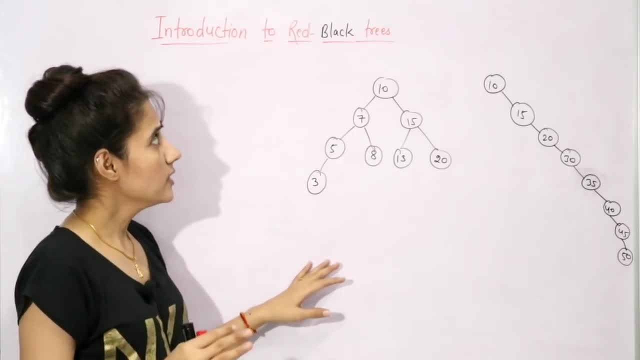 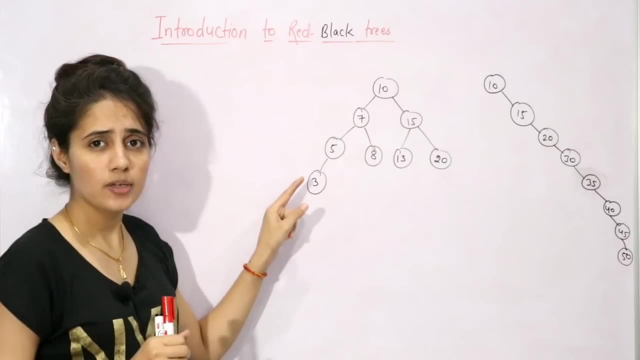 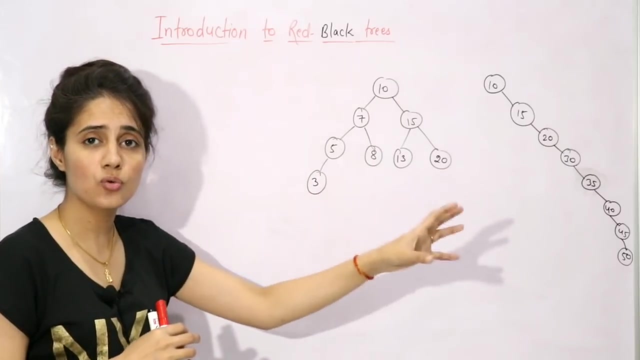 video in the side button. fine, Now what is a binary search tree? see in the. in that case, always the left subtree of a node would contain the value less than that node And the right subtree of the node contains value greater than that node. See, if you say that, see. 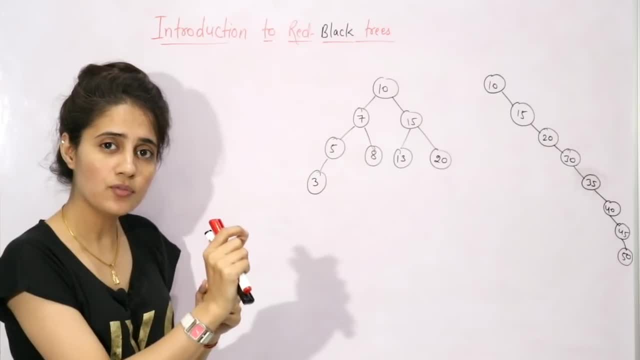 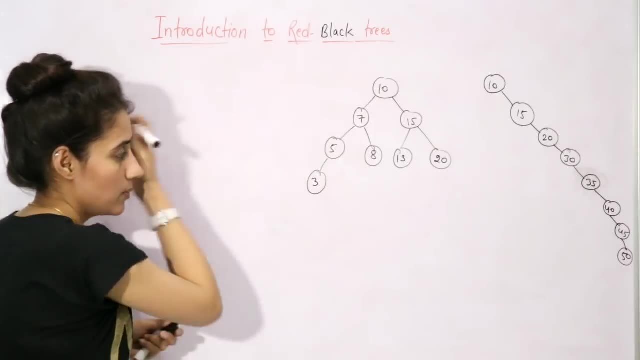 somewhere it is written that that left child of a node is having value less than that node and right child is having value greater than that node, If you follow that property. in that case- suppose here I'm drawing that BST- this is a node. it means left child of this should be less than 10.. 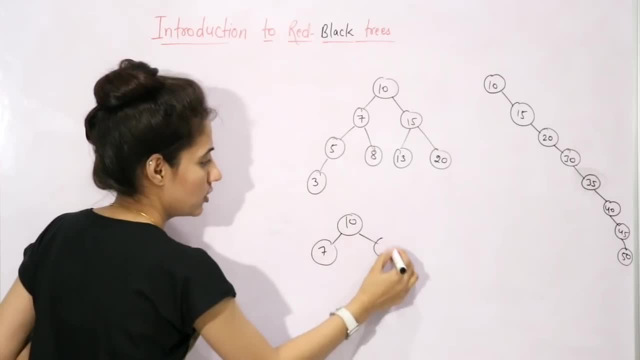 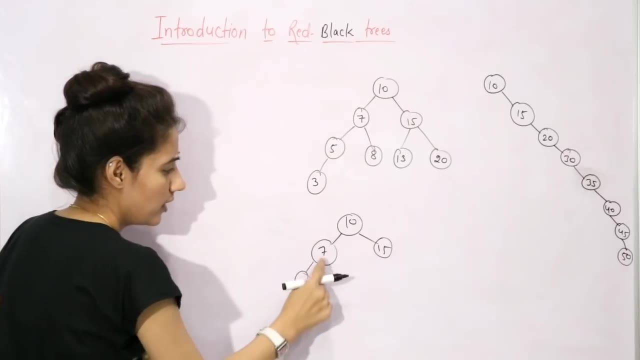 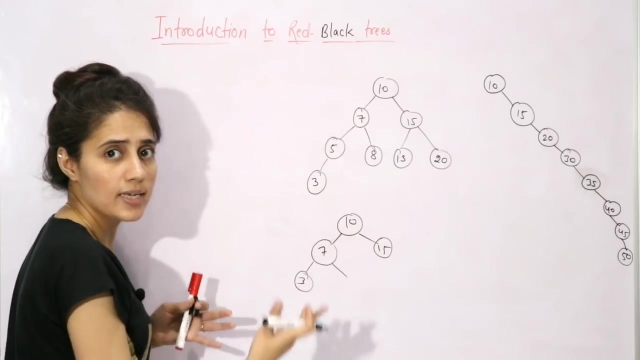 Suppose I'm taking seven, right child should be greater than 10.. Suppose I'm taking 15. Now this property is applied in all the nodes, on all the nodes. Now for seven, left side child should be less than seven. Suppose I'm taking three, right child of seven should be greater than seven. Now, 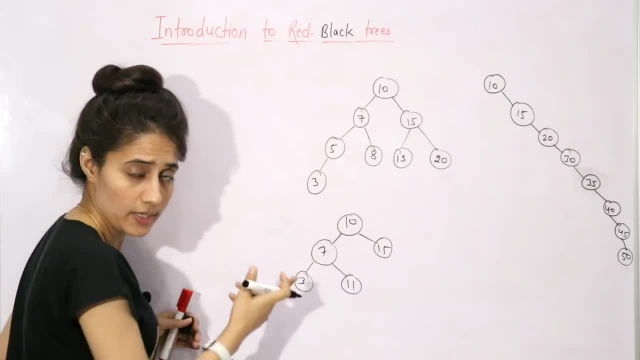 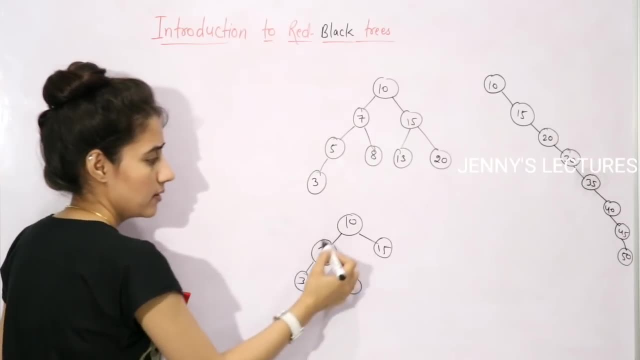 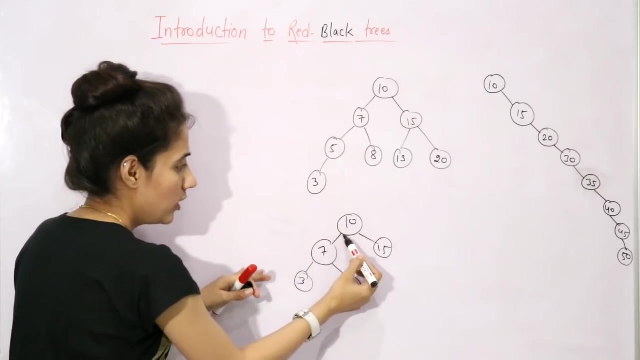 I'm taking here 11.. But is this a BST? No, it is not a BST. You should say that the left subtree, because he's 11 is greater than seven, but 11 is greater than 10 also. But to the left of 10, the value should be less than 10.. It means this is the left subtree for this. 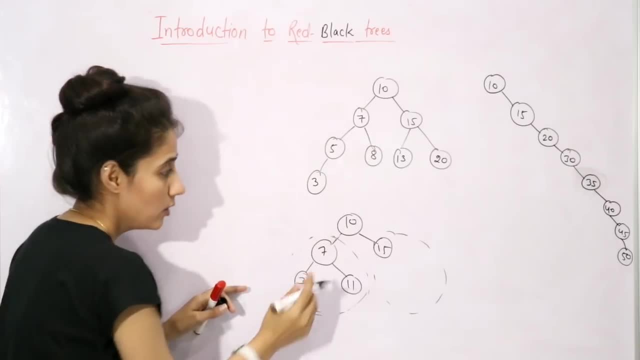 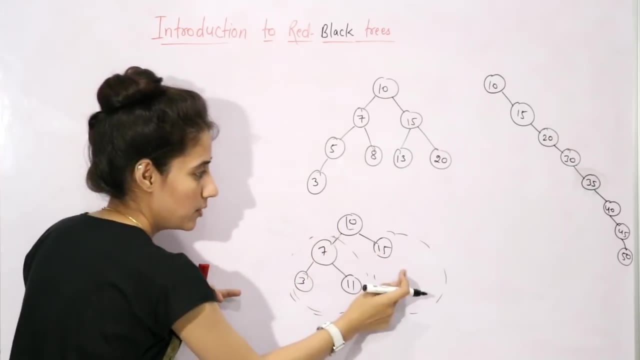 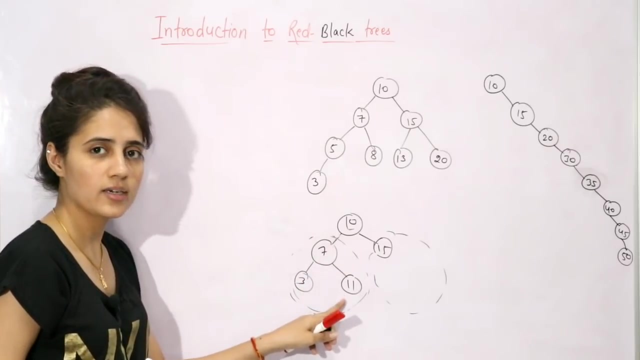 10. This would be the right subtree for this 10. Right, So in this left subtree, left left subtree of any node should contain values less than that node and right subtree should contain values greater than that node. So it's better to say that, rather than left child and right child, 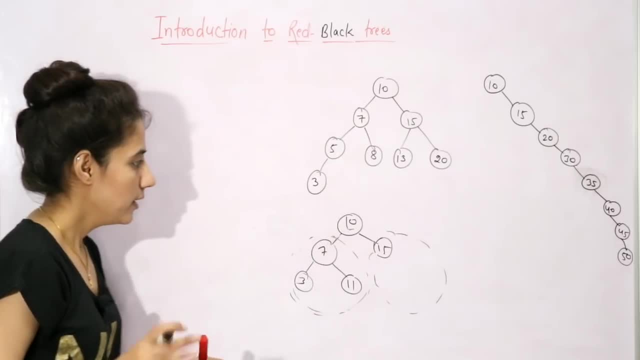 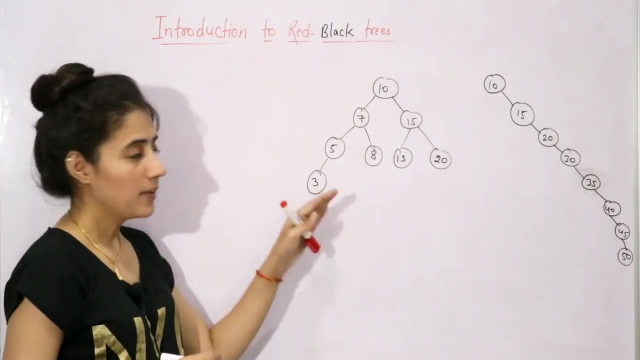 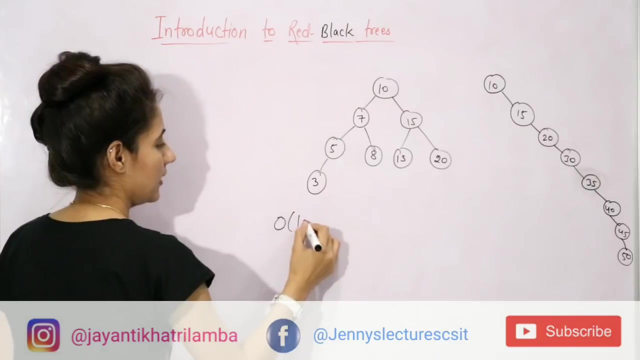 it is better to say left subtree and right subtree. Fine, Now see, I'm taking these. both are binary search trees. Now, as we know that in binary search tree the searching, or you can say insertion and deletion, is going to take order of log n time. 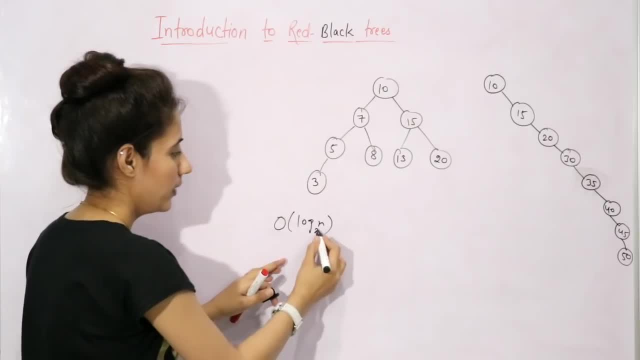 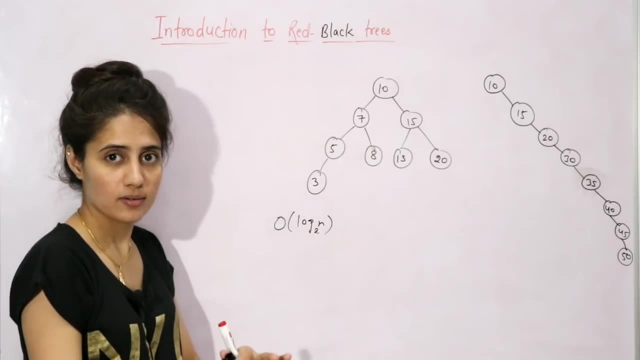 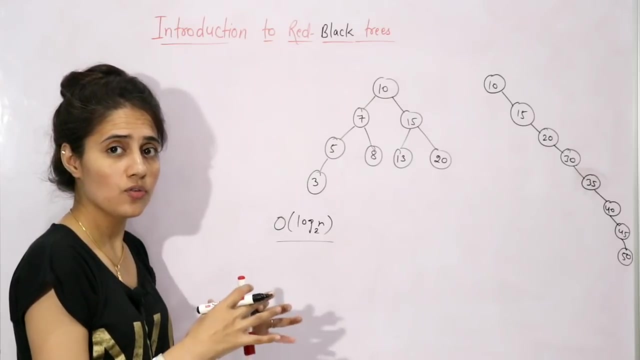 in average case log two, base two and n in average case. in best case it is order of one. in worst case it is order of n right. in average case it is order of log n right. So we can say the searching of any data in binary search tree is going to take less time. That is. 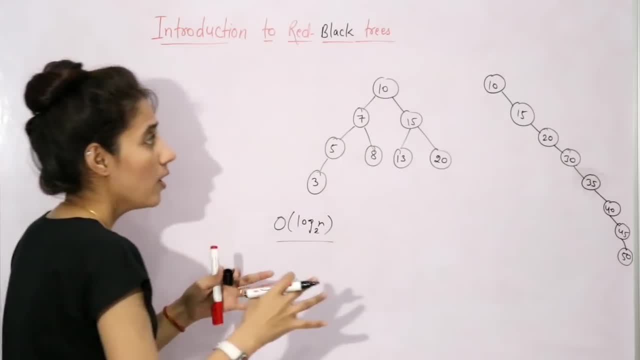 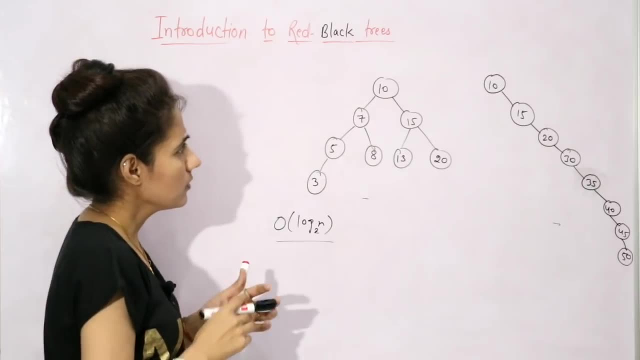 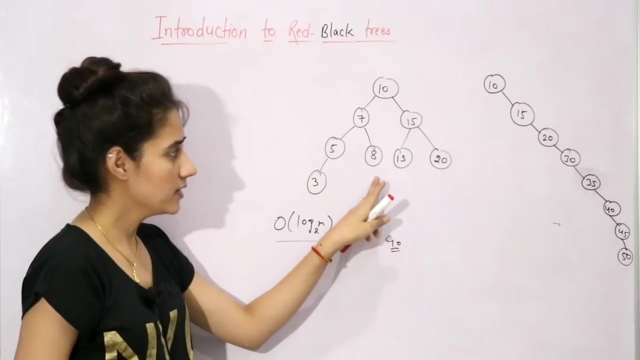 why? obviously we are using tree data structures, right? How see? suppose I'm taking. this is one BST, this is another BST, two types of BST we have now see if I'm I want to search for a number- 90 in both the trees. in this case, 90 means we will compare with the root. 90 is greater than this. 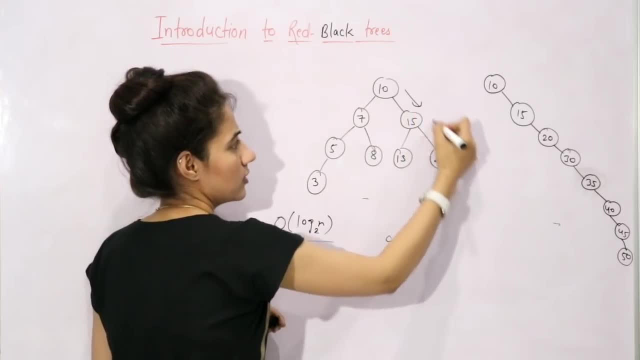 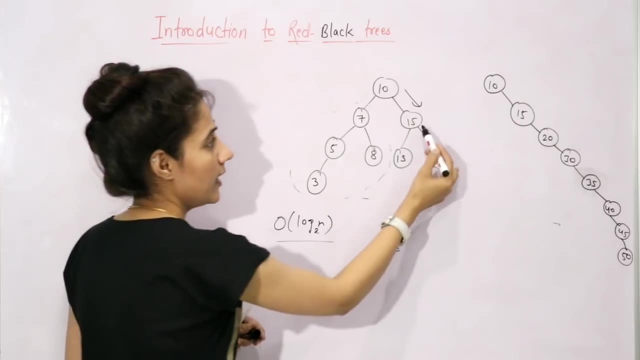 root: greater than 10.. So we will go to this path. this root means we are not going to check all these elements right Again. 15- 90 is greater than 15. So we will go to this root. we are not going to compare. 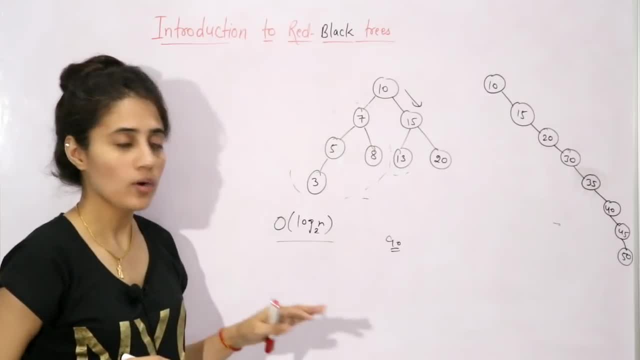 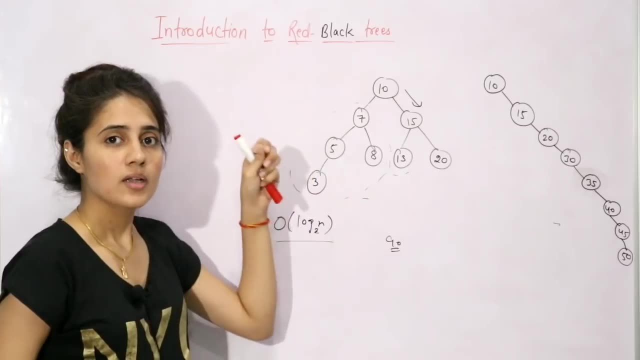 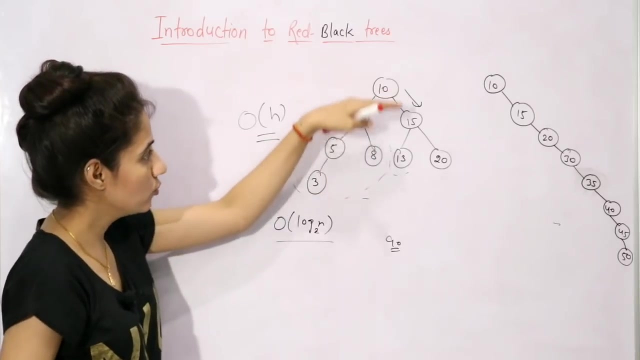 this with this 13.. That is why here we need not to compare this element with all the data present in the BST. that is why the searching is going to take less time, or you can say it is going to take order of edge time. The time complexity would be according to the height of the BST and basically it is what height? 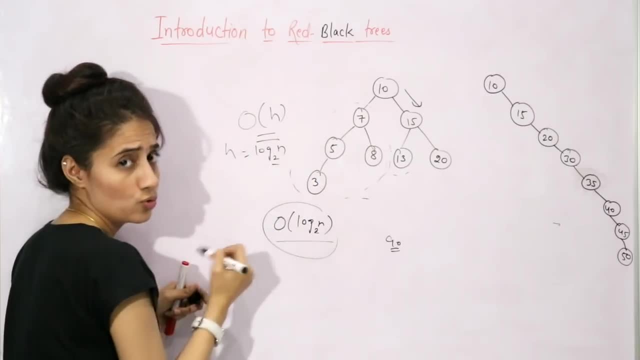 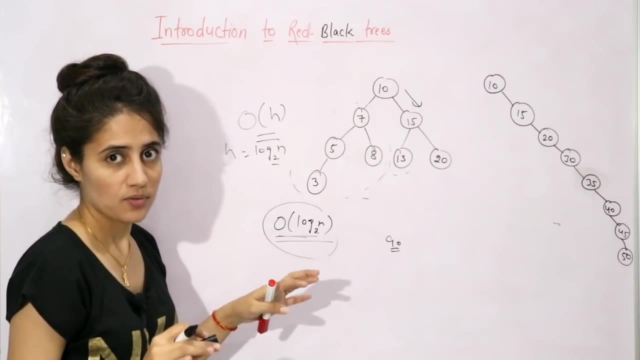 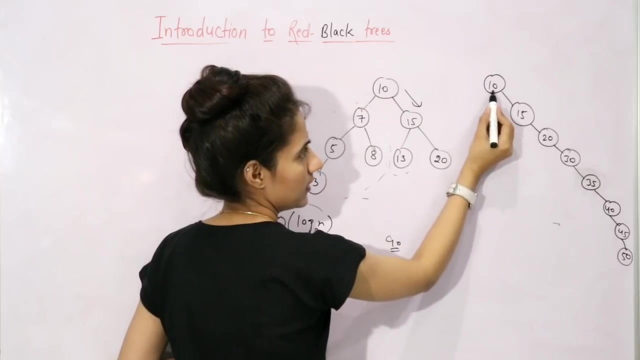 is log n and base is two. So that is why time complexity would be: order of log n, two, right, This is the average case. you can say: fine, Now in this case, suppose I'm searching for 90, in that case, greater than 10, we will go to here. greater than 15, there there, then, there there. 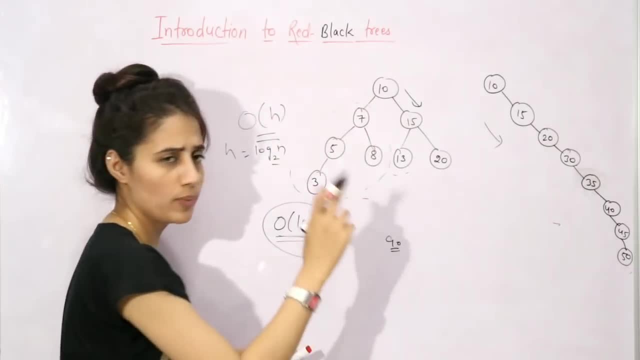 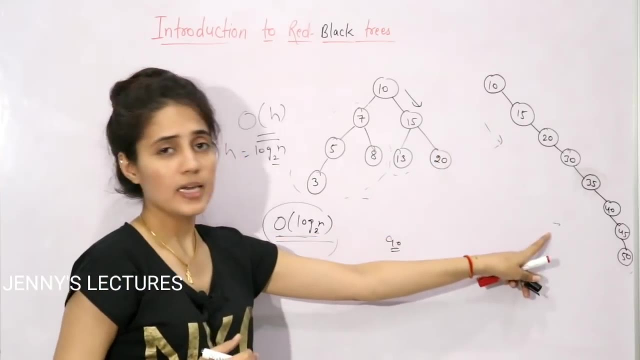 there and then after that it will Give you that the 90 is not present in the tree. But here the time complexity would be. you have compared this element with all the elements present in the BST, So it is equal to order of n. 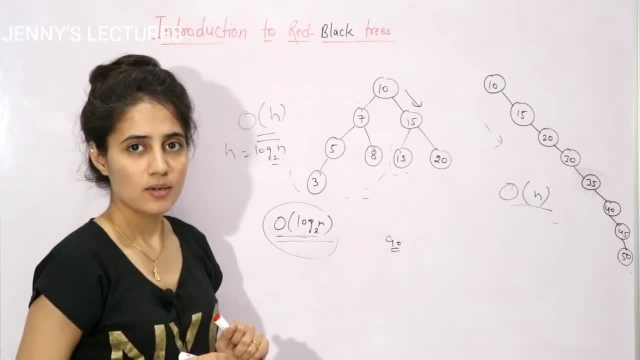 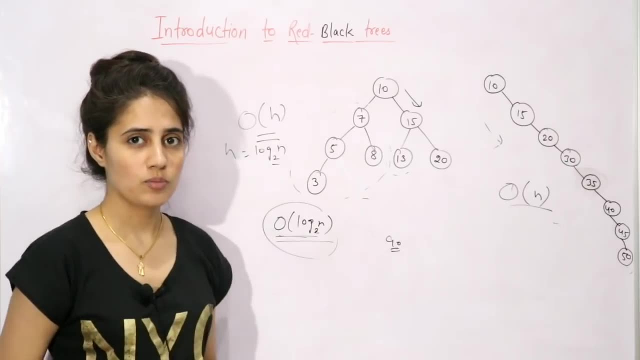 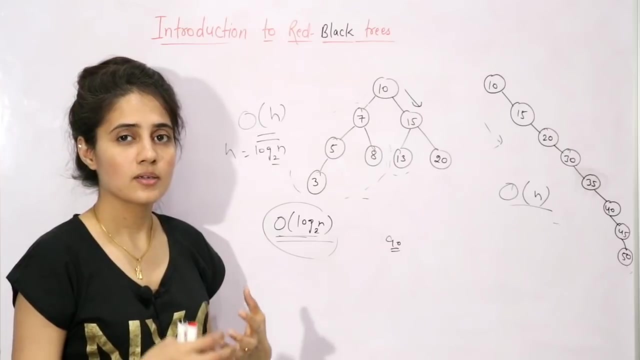 So this is the worst case, right, And we want that the time taken or the time complexity would be as less as possible. So that is why, rather than this- this is what a right skewed BST- We want that the tree, the BST or the tree should be balanced. See, this is what a balanced BST you. 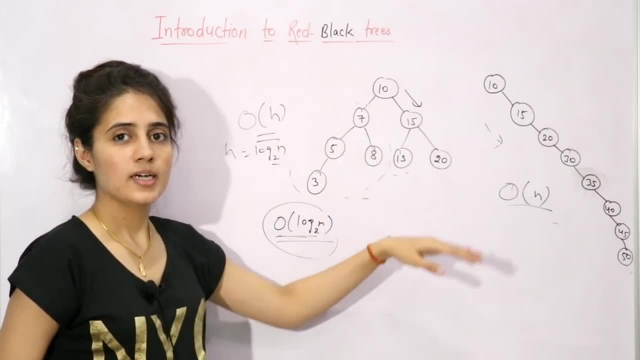 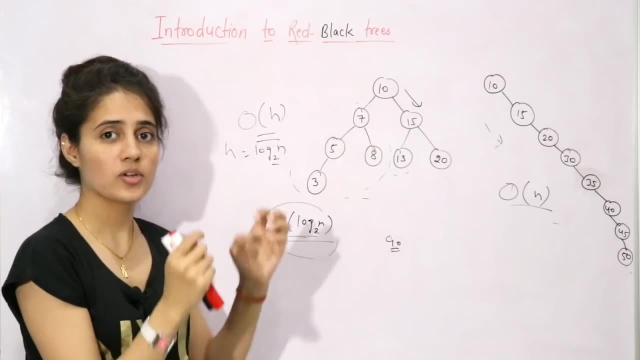 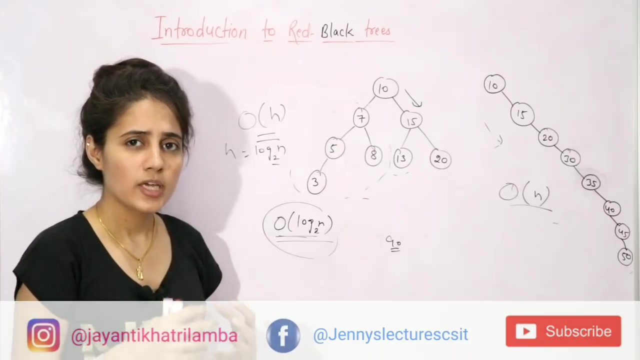 can say So whenever we will insert the data. we all we always want that the tree would be balanced so that all the operations- like insertion, deletion, deletion, searching, find, minimum and maximum, all these operations should take, all these operations will take time. complexity. order of log n. 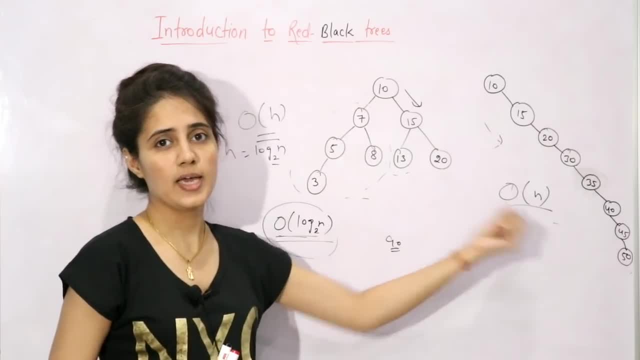 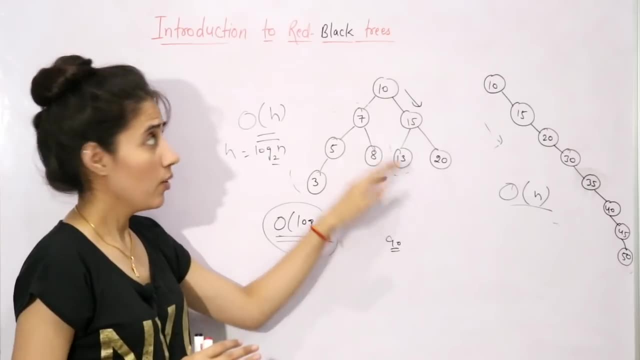 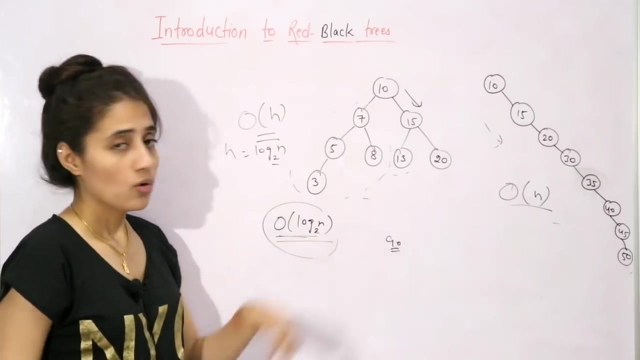 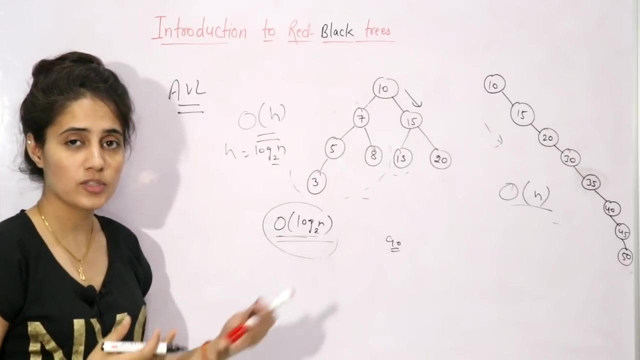 that is very less than order of n. fine, now, okay, we will need. what a balanced tree? now, and red black tree is also a self-balancing binary search tree. but now you can say that also, we have a tree that is avl, this is also a self-balanced, or you can say a height balanced tree. then why we need? 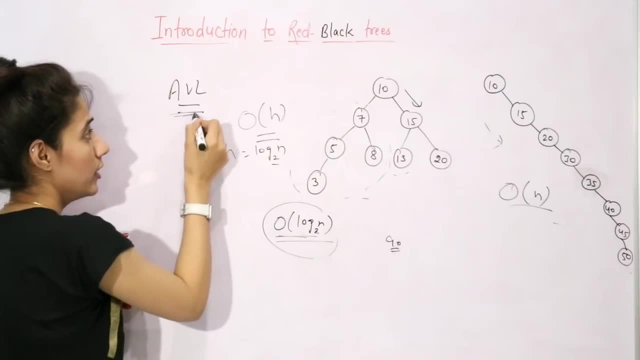 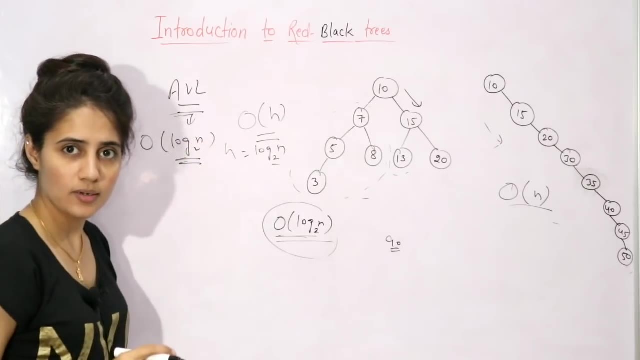 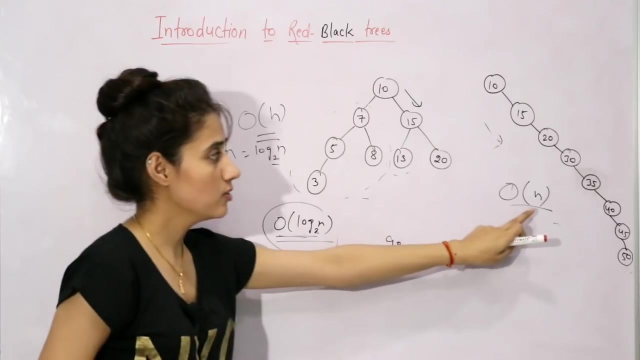 red black tree. right because in avl tree also. it also guarantees that the time complexity would be order of log n. right in all the cases, in worst case, in best case, in average case, in bst. in worst case it is order of n because the bst can be left skewed or right skewed, something like this: 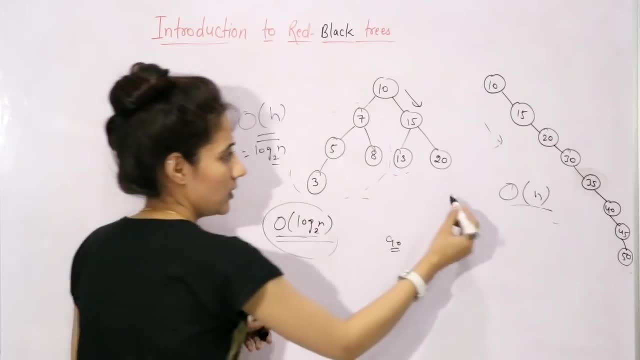 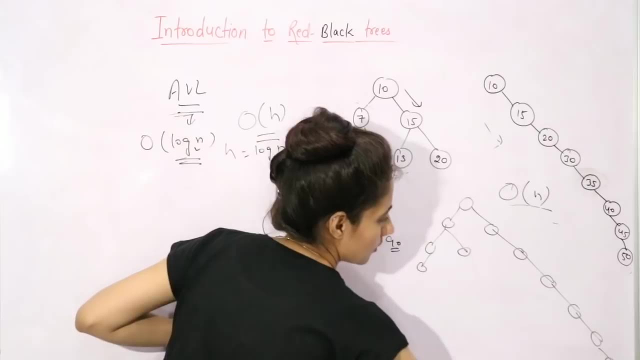 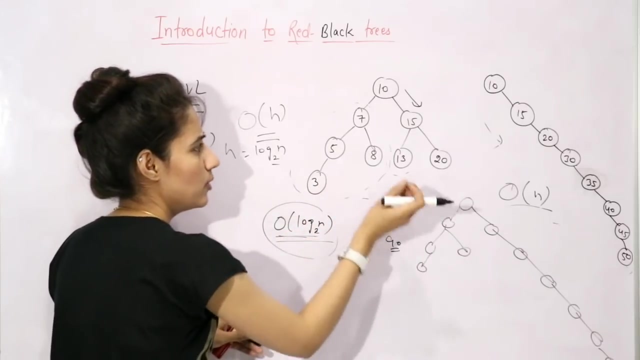 or it may be between this, this, this and this, suppose something like this: here we have bst- this tree, so this is also a bst. here you can write down the numbers according to the bst that follow that rule. only this is between this and this. this is not a left or right skewed. 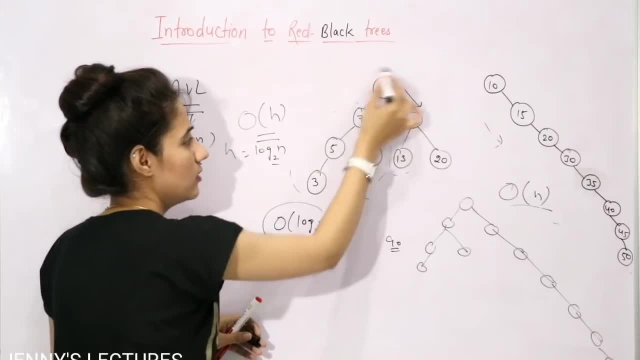 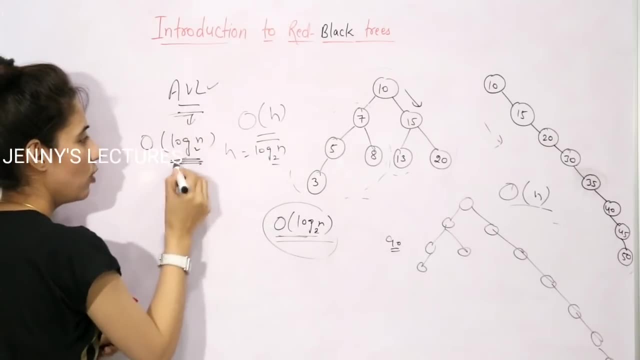 and this is not a balanced tree, right. but we want that the tree should be balanced so that the time complexity would be less order of log n. but avl tree guarantees that the time complexity would be log n only because this is what height height balanced tree. so why? 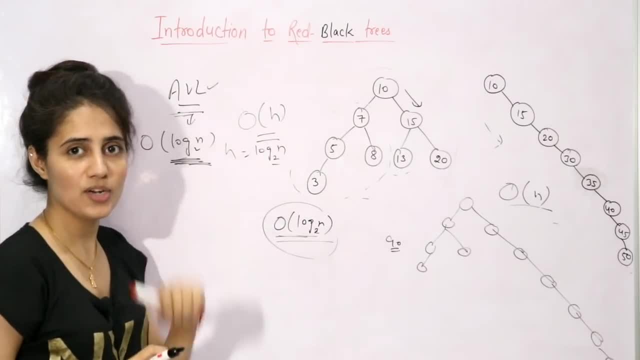 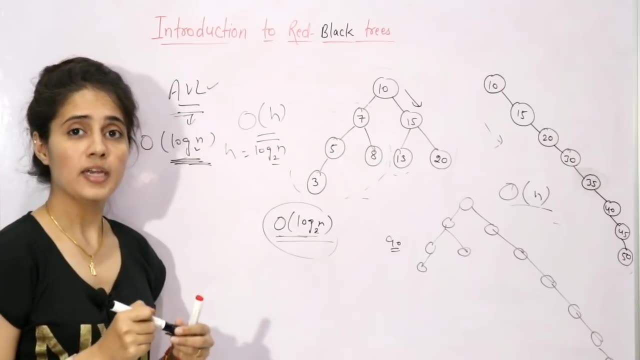 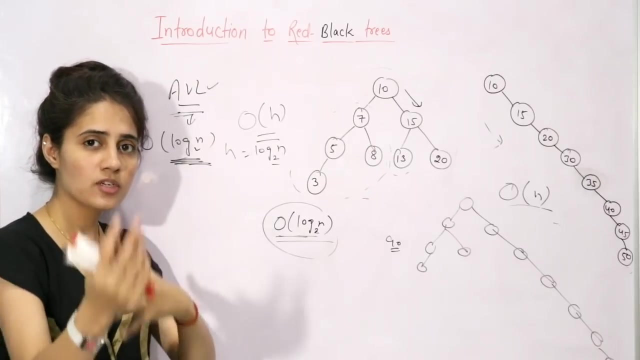 we are using red black trees. how red black trees are different from avl trees. see now. main difference is what in avl tree you need to do many rotations sometimes if tree is very large, so maybe you require more than two, three, four, five, six or many rotations to balance that. 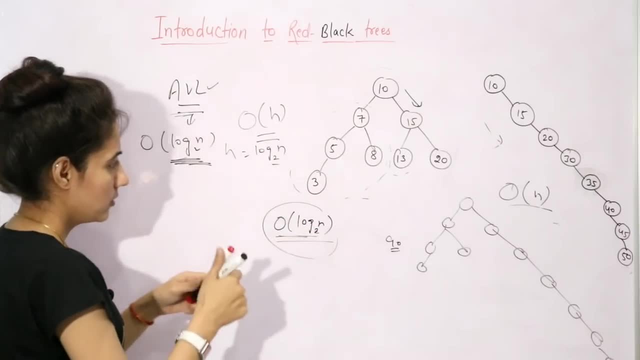 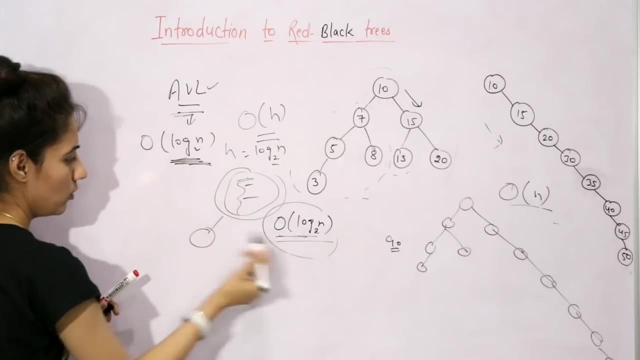 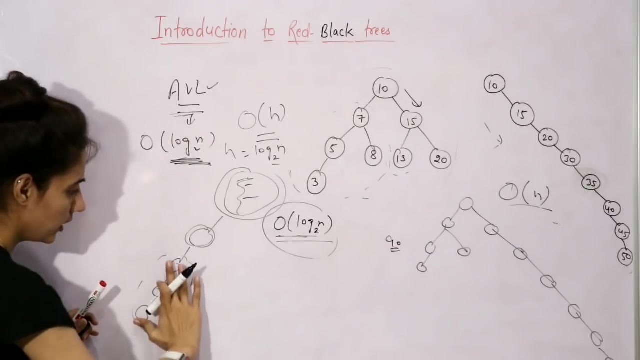 tree. suppose, at this point of times, tree is something like this here. this is a tree having multiple nodes, this is some. there is some node we have and at this case we need to do some rotations. so after rotating this, after doing this balance- suppose this tree's the upper tree, is what unbalanced? so 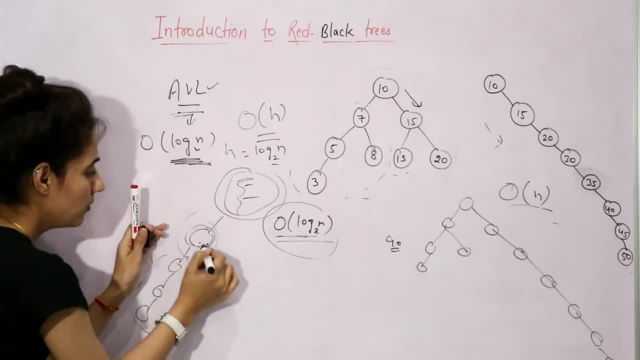 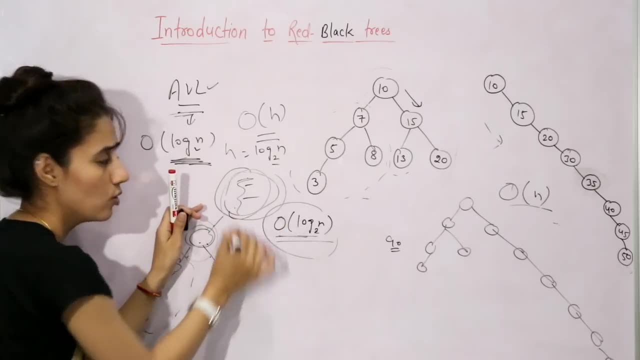 so you need to do rotations at the this part. after balancing this part. suppose there is the tree is unbalanced at this part, at upper level, so you need to balance here also, right? so So we don't know how many rotations would be required. Maybe we require the rotation up to the root node, right? But in red-black trees maximum two rotations would be required and the tree would be balanced right, And sometimes even the rotations would not be required and recoloring would be required. Recoloring means, as the name suggests, the nodes would be either red or black. 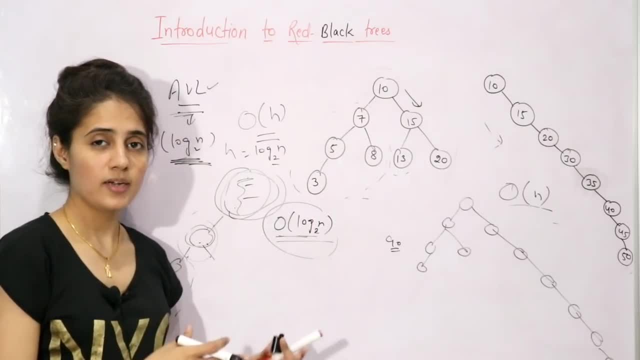 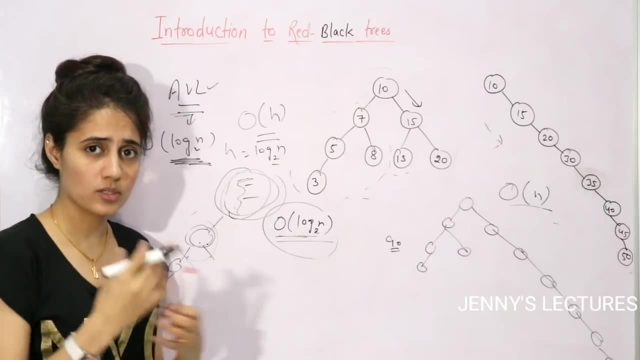 So you need to change the color only. If the node is red, just change it to black, Something like this. we will discuss these rules in the next video when we are going to discuss the insertion part. right, So sometimes only recoloring would be sufficient. 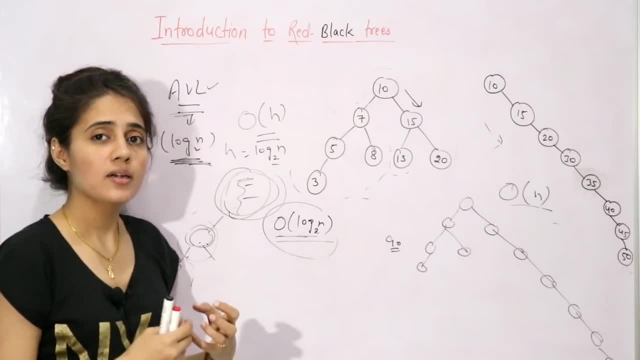 No rotation would be required. And if rotations are required, then only you know. you can say maximum two rotations would be required. Rotations plus recoloring may be required, but not more than two rotations. So very less rotations would be required. 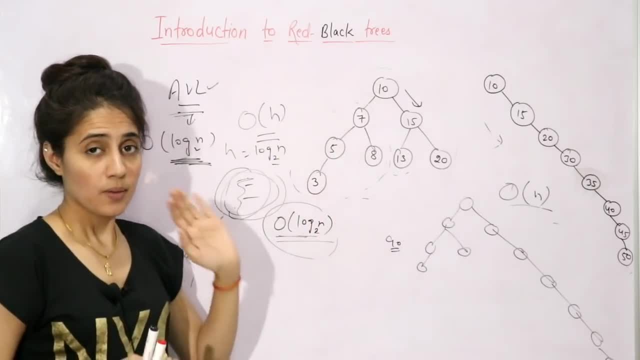 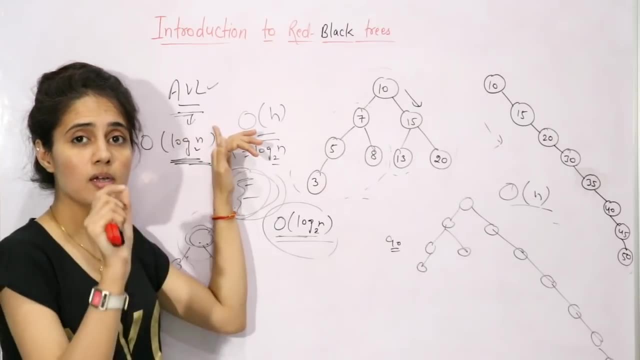 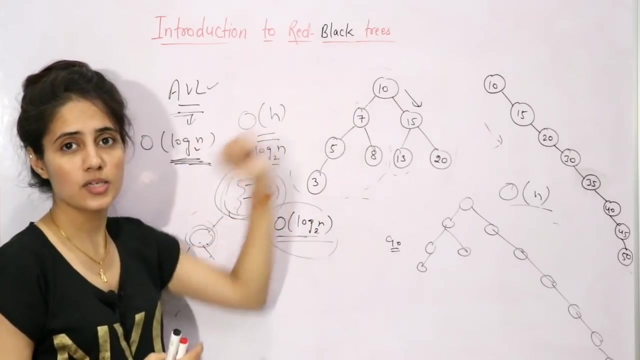 In a red-black tree is to balance that tree. But see, red-black tree is, you can say, a roughly height balanced And avial tree is strictly height balanced tree. Or you can say avial tree is more balanced than red-black trees. 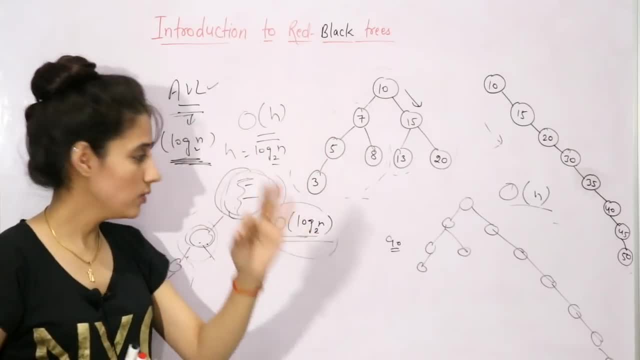 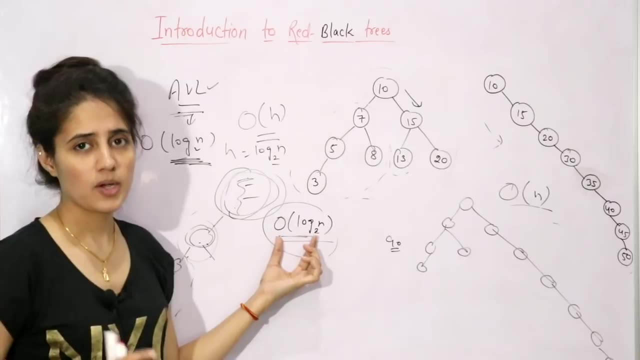 But red-black trees guarantees you to give the time complexity order of log n for all the. you can say searching, insertion, deletion these kind of operations, And that's it. That's exactly we want The time complexity would be this one right. 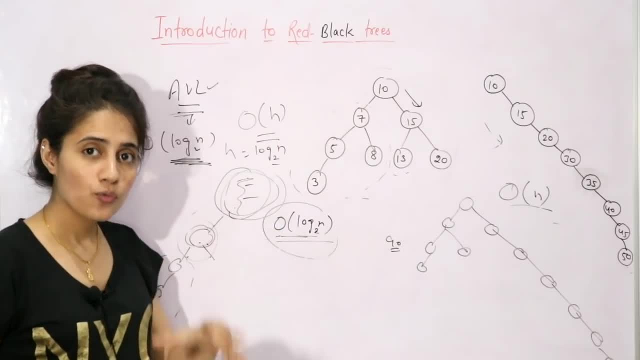 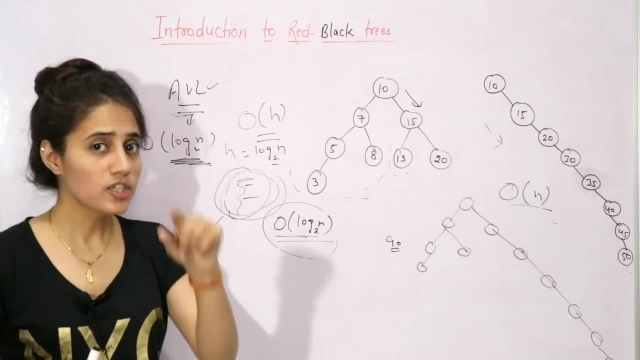 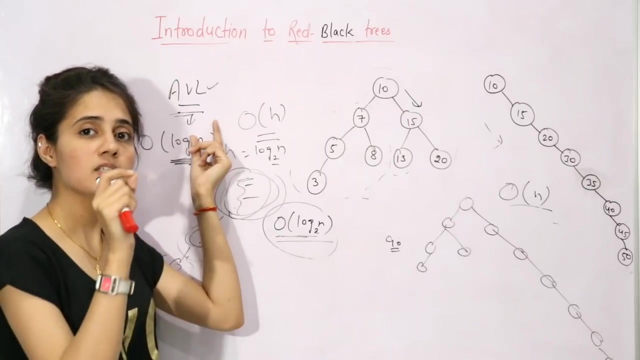 So we can go for red-black trees In the case when you are you are going to perform insertion and deletion operation very frequently. See, searching is faster in avial tree because it is strictly height balanced tree, But insertion and deletion is faster in red-black trees because here we require few rotations. 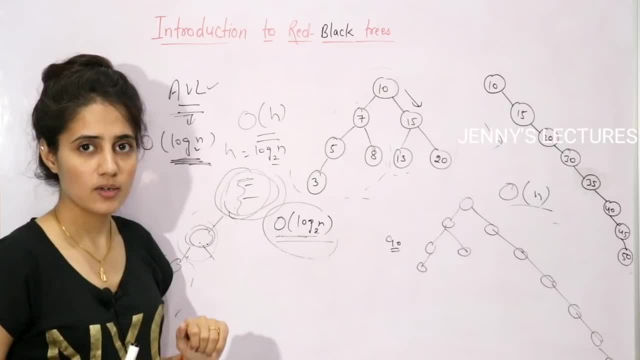 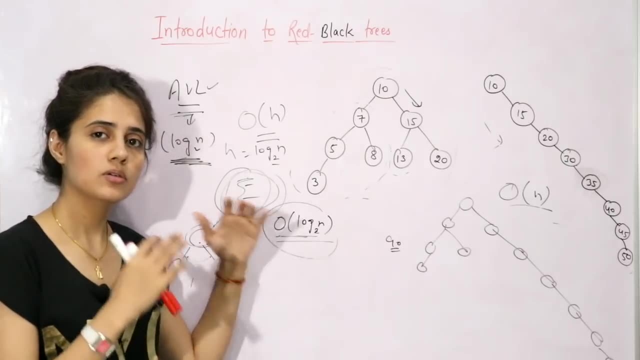 And in avial trees we require many rotations, Right? So depends on the situation, depends on the operations you want to perform on the tree. we are going to choose the trees. It's not like that: red-black trees are best and these are not good. 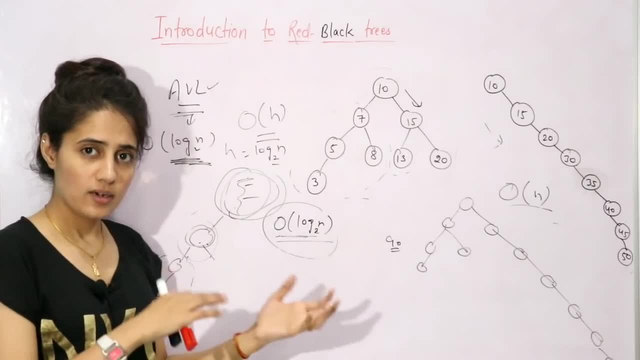 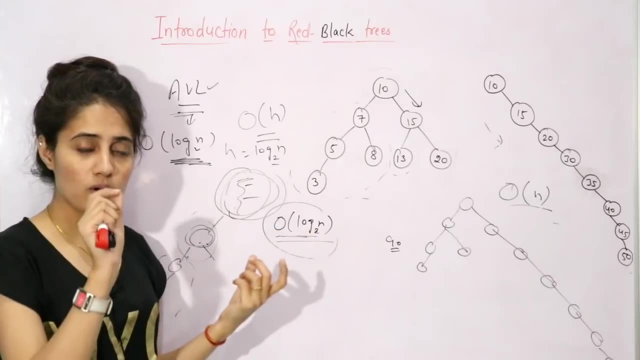 Right, It depends on the situation. Fine, In the separate video I'll discuss the difference between avial tree and red-black trees properly. Right Now, I guess you have got that why we need red-black trees. Fine, Now we will discuss and how red-black trees are best. 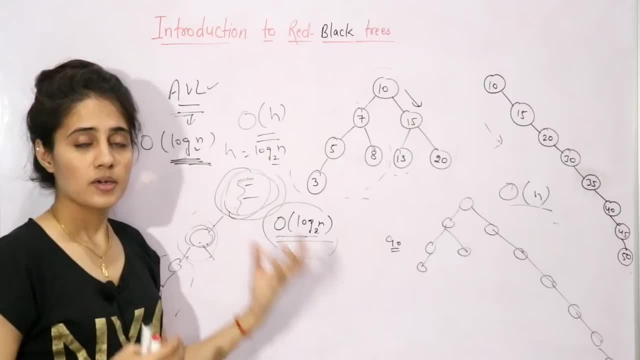 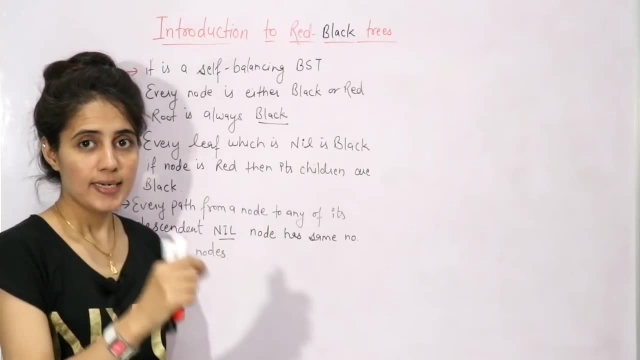 Right, Because red-black trees are different from avial trees. Right Now we will discuss what is red-black trees and properties of red-black trees. So these are some properties of red-black trees. See, it is a self-balancing binary search tree. 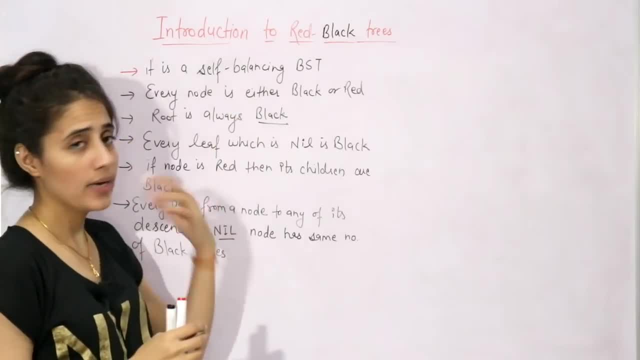 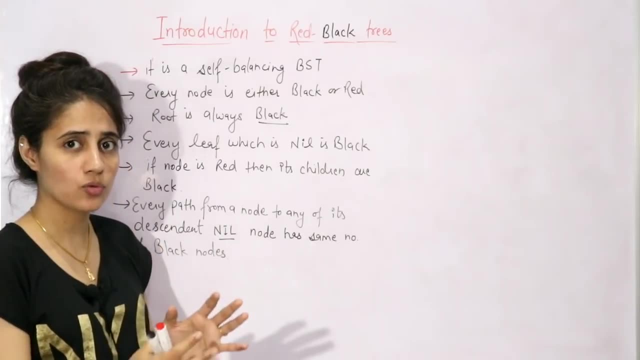 We have discussed what is binary search tree and what is. self-balancing means it is going to balance itself By doing some rotations or recoloring. That thing we will discuss in the next video. The rule of rotation and recoloring- That thing we will discuss in the next video. 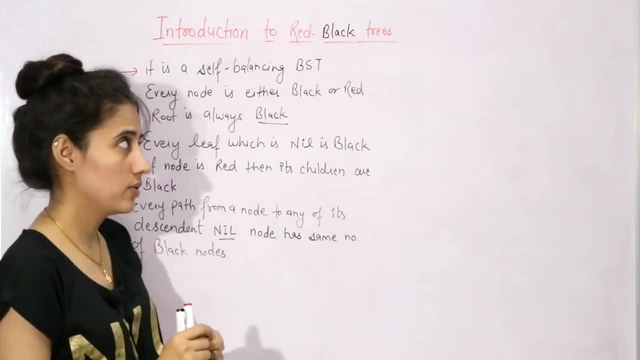 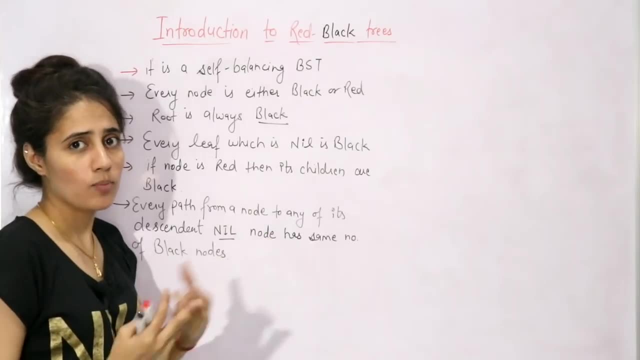 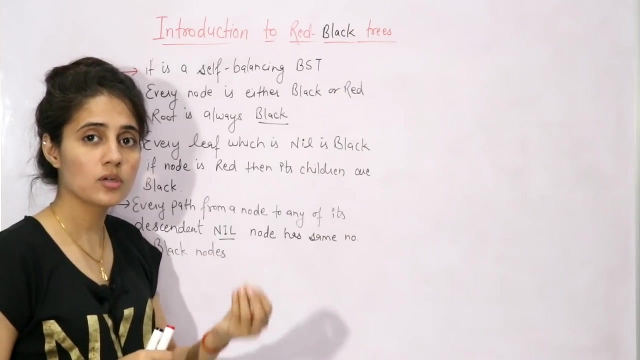 When we will do the insertion in the tree, When we will do the insertion in the red-black trees Right Now. next is, obviously it is a red-black tree, So every node is either red or black. Right, It means every node is having a special bit which shows the color of the node. 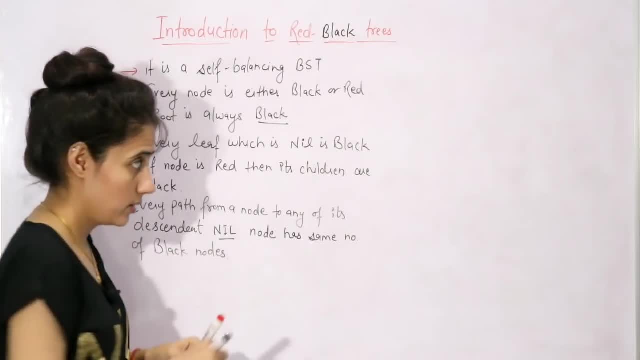 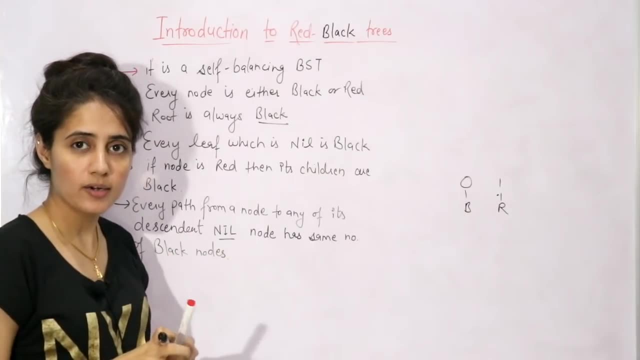 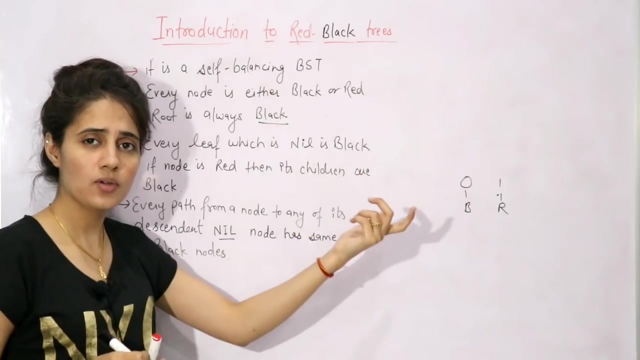 Right A one bit. You can say: 0 means black and 1 means red. Only one extra bit would be required with each node And rather than this bit, each node is containing what? Obviously, the node is same as binary tree we have discussed. 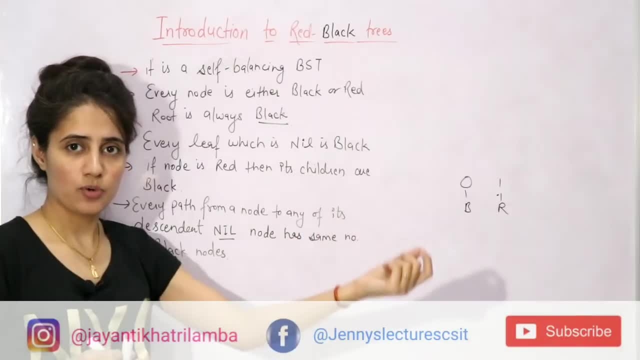 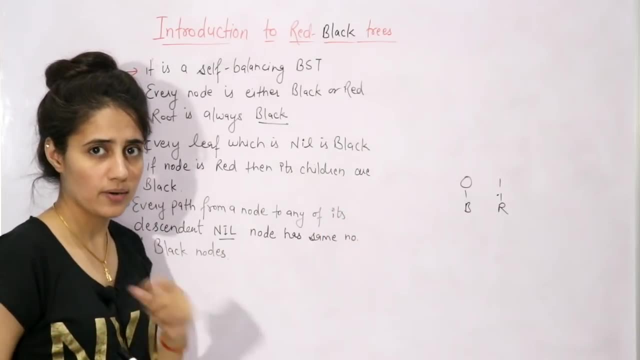 The key, or you can say the data: left, pointer right, pointer Right, Plus this. also One bit for storing the color of the node. That is also mandatory, Right. How to write down the node, that structure of the node, that thing we will discuss in the implementation part. 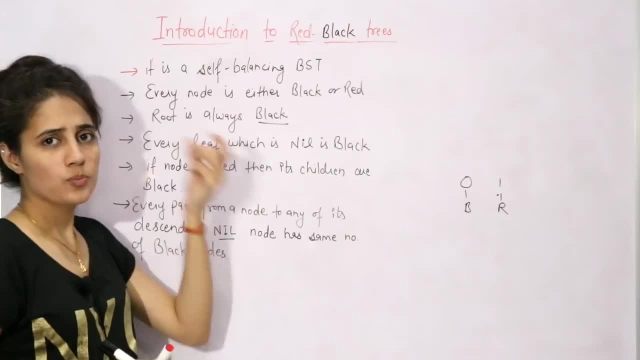 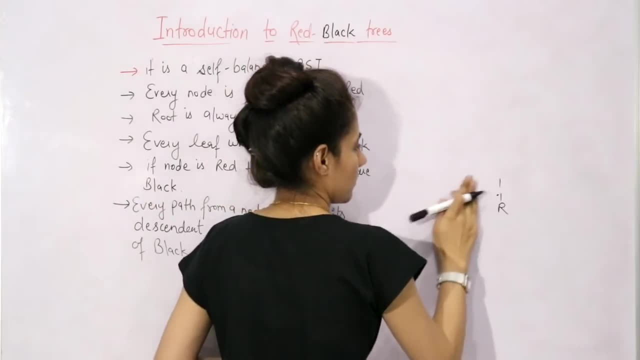 Right Now. next is what See, root is always black. Or you can say: the head node is always black. So now, in this case, see: Suppose this is a tree, This is- I am taking root node. Obviously, we have one node only, so that would be the root node. 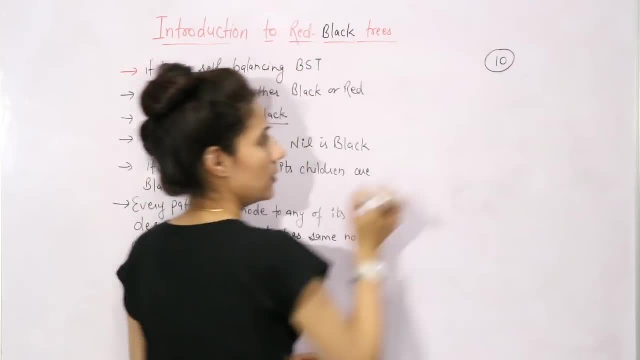 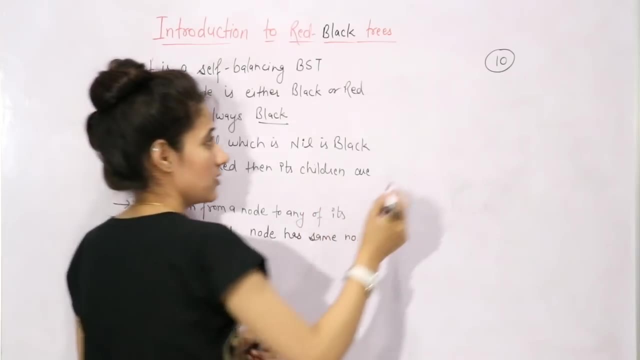 So this is always black, Suppose I am taking here the number 10. Right, Or you can relate it with real life example. Obviously in the tree we have something like this 10. Here also we have some. So these are what. 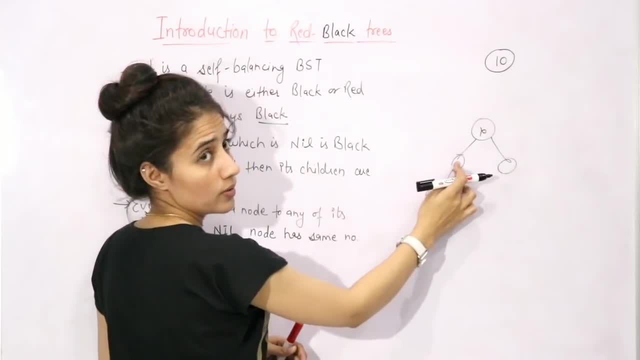 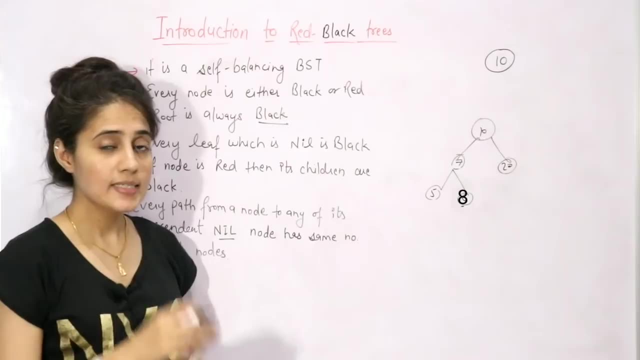 Child of this 10. And these are child of this 10. Right Suppose: here I have 7., 5. So for these, this is the grandparent, Or you can say the head of the family, And see when a person gets angry, then you can say: the face of that person becomes red. 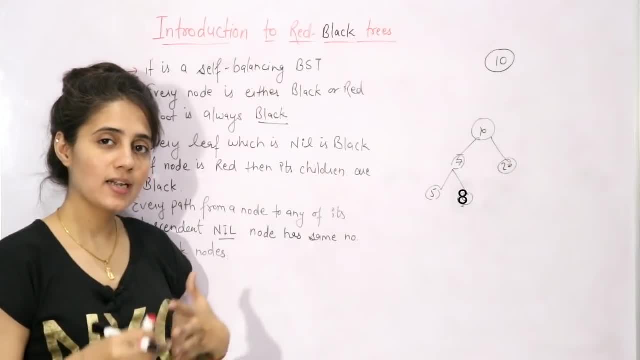 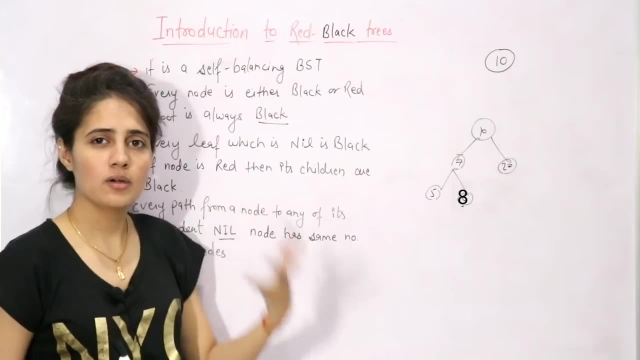 Right. And we consider here that if a person is calm or cool, then the face of that person is black. So the head of the family always try to remain calm Right. Or you can say the grandparents, You can relate it with- that they do yoga and all. 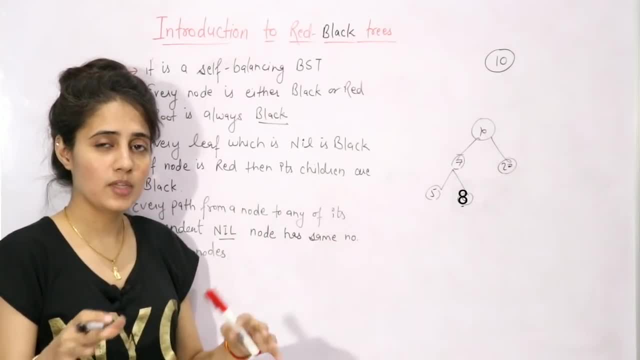 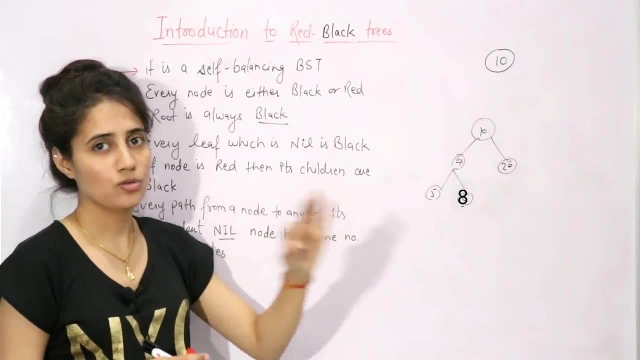 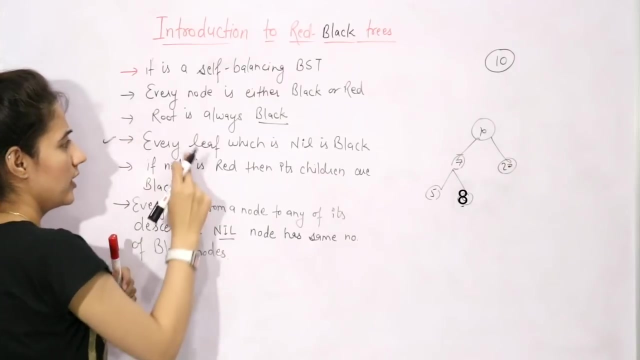 And that is why they always remain calm. They usually don't get angry. That is why the root or the head node will always be black, Not red, Right Now. next is what Every leaf See. this property is very important. Every leaf which is nil is black. 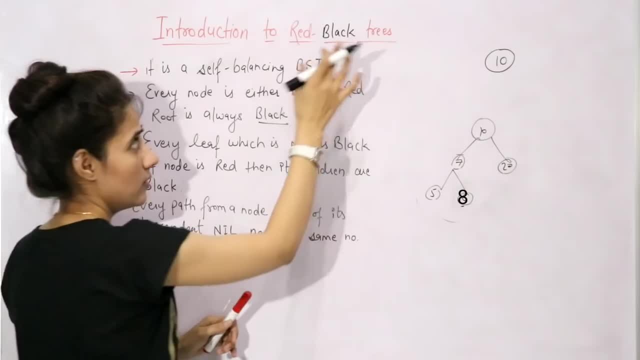 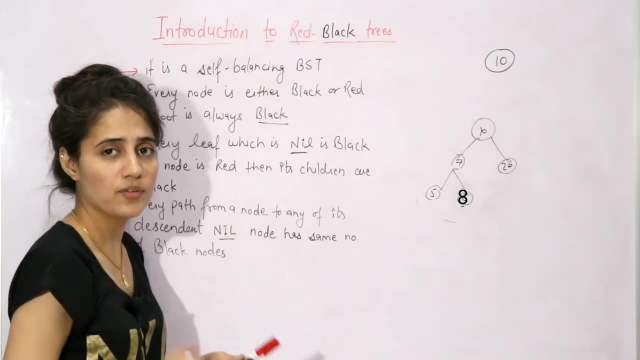 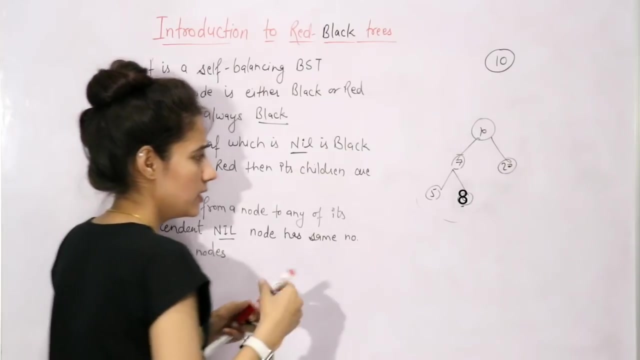 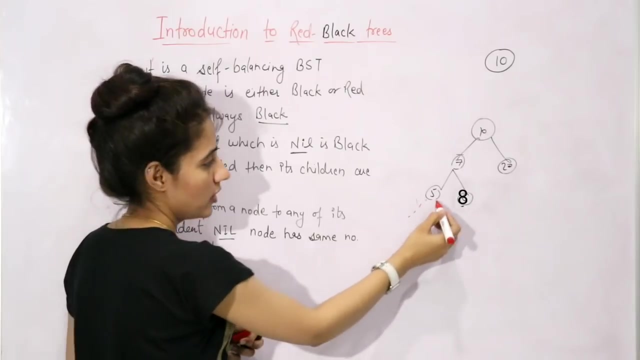 Here in this case, if you are not considering red black trees, this is a binary tree. Here the leaf node are this, this and this. These are not having any child node. But in red black trees what we consider is See here, if this is a node, means this is the leaf node, it is having no left child, no right child. 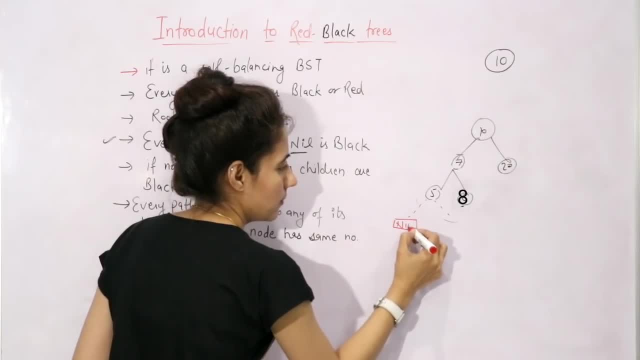 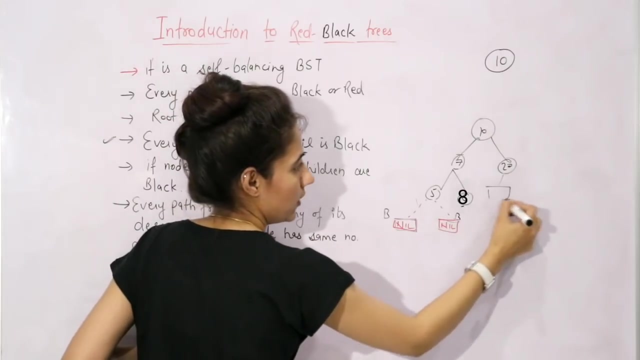 So here we consider nil, This is nil, this is nil. And see, obviously this color is what it should be: black, Not red, it should be black. So every leaf which is nil is black. So it is also having no left, no right. 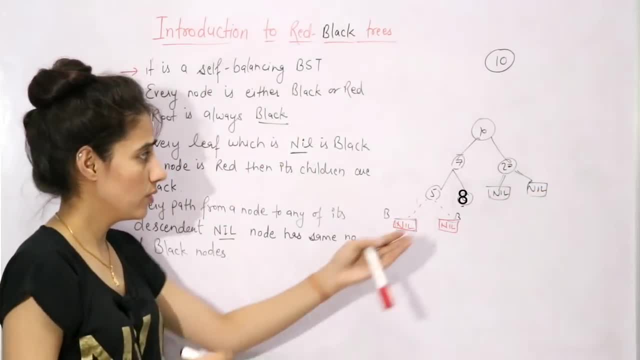 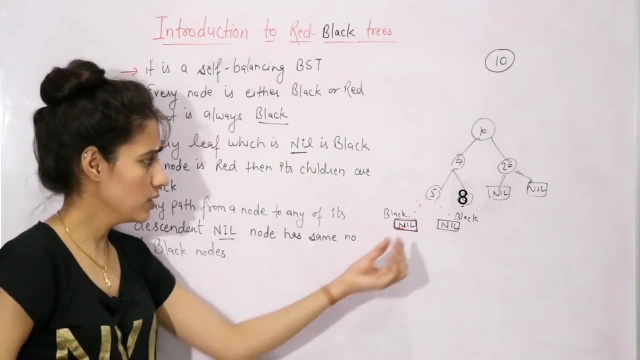 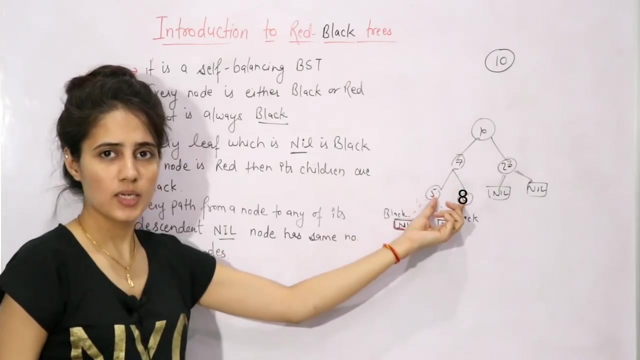 So it is nil, it is nil. So we usually draw red black tree, something like this: See, we are not going to consider these nodes as a part of the tree. This is what external nodes Right. Generally, we don't count these nodes in this tree. 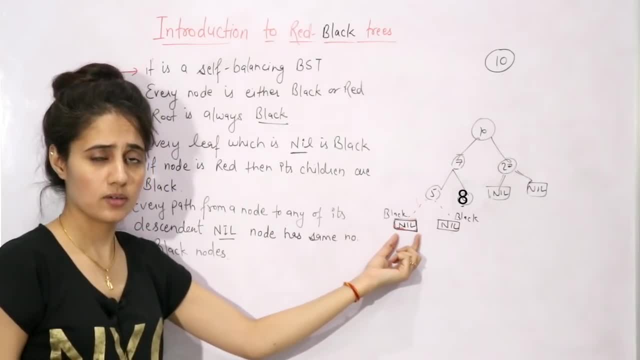 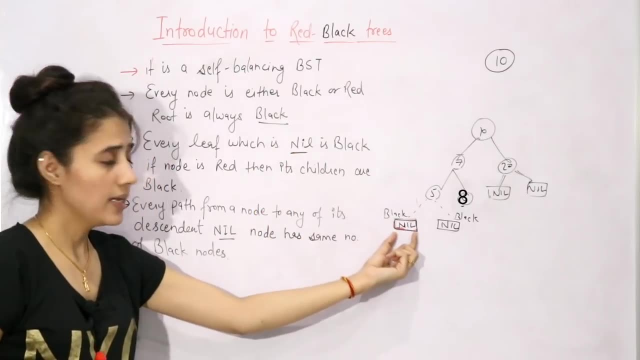 But these are helpful when we will insert nodes And delete the data from the tree. Fine, So now every leaf node which is nil is black. Which is nil is black. It is not like that this is leaf node and this would be black. 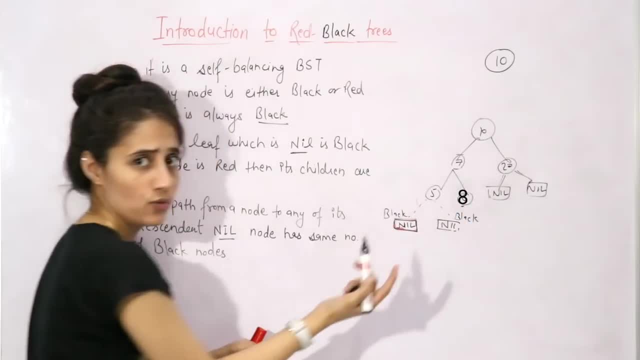 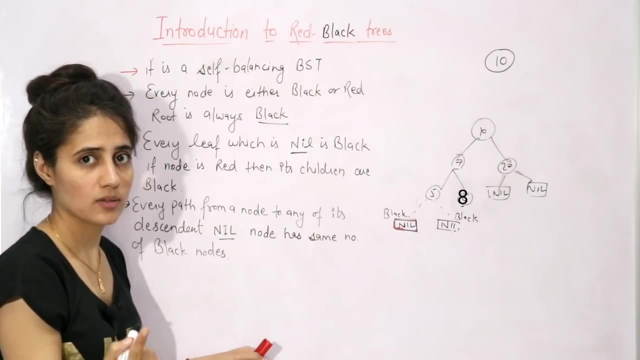 No, Here we are. not consider these as leaf node. Leaf node would be these nodes, The nil nodes. These are considered as internal nodes of the red black trees. Right, This thing you need to take care. So now suppose this is a tree. 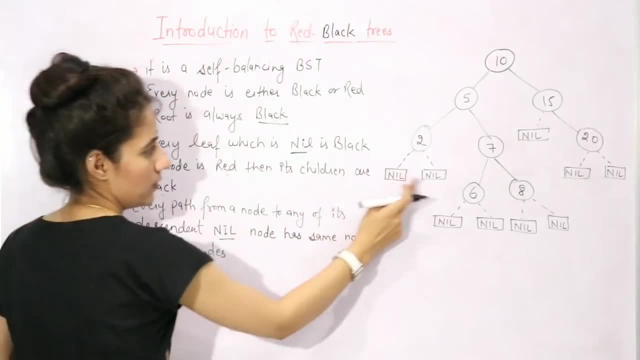 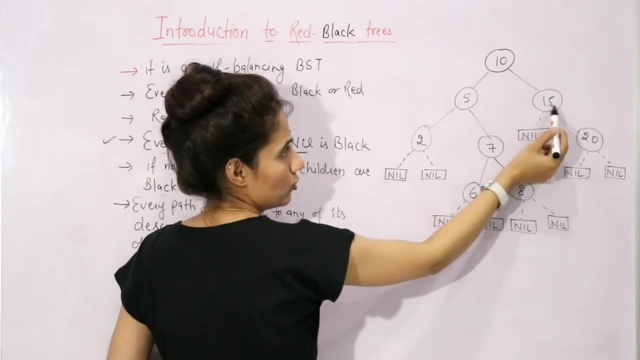 Here this root is always black And we have taken these nil nodes. Every leaf which is nil is black, Right, So see here also, this node is also having no left child. It means basically we can consider it with a pointer, Left pointer, right pointer. 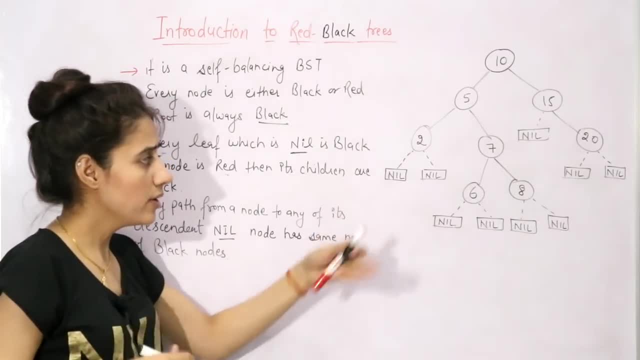 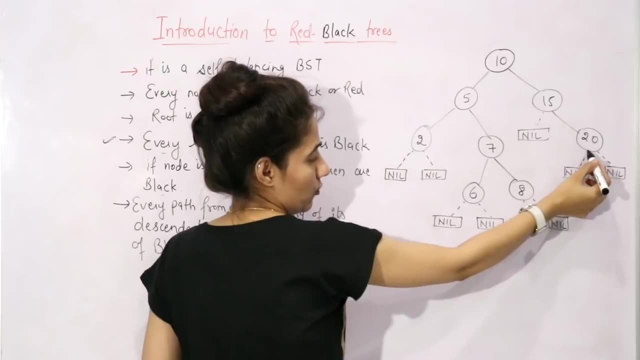 Those are null pointers. So here I am drawing these as a node. that is nil, nodes Right. Simply you can say So. here also, the left is nil For 20, both left and right would be nil. So these nil would be black. 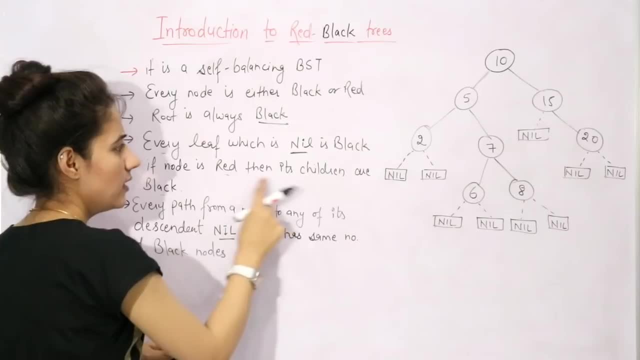 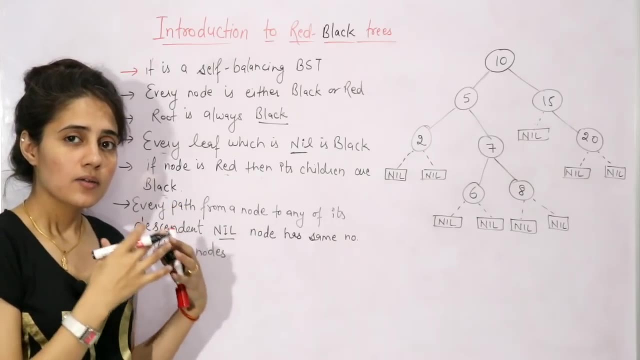 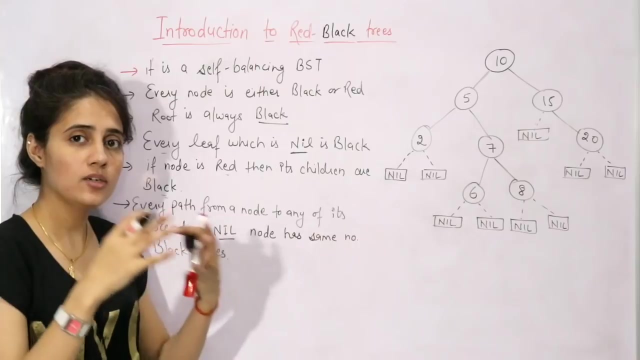 Right Now see. next is: if node is red, then its children are black. It means here you can, in another term, you can say There should not be no red red parent child relationship. Or you can say that no adjacent node can be red. 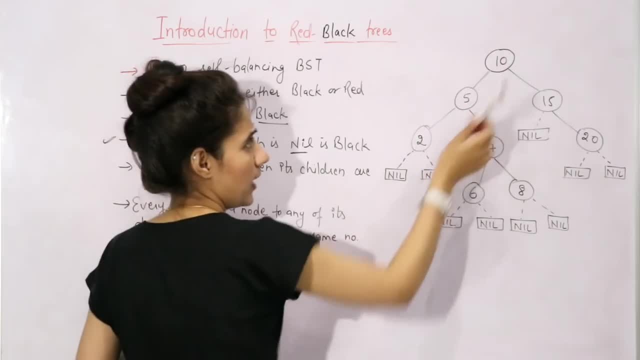 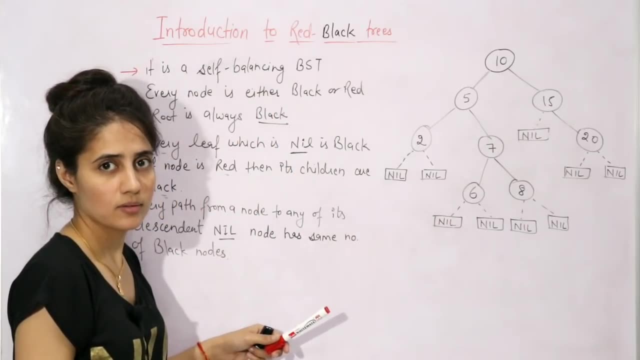 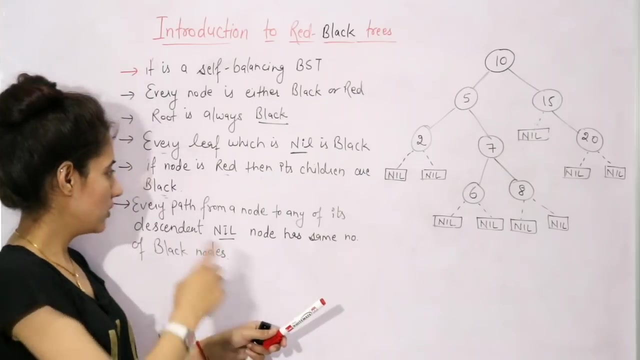 Something like this: See, this root is black Right, So this and this can be black, can be red Right, Because constraint is only on the red nodes, Not on the black color, On the black nodes. constraint is this one, that thing we will discuss. 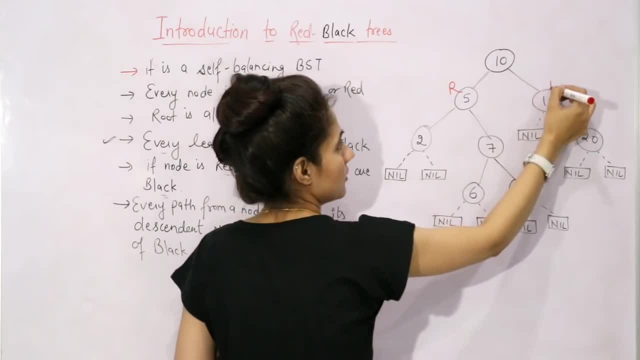 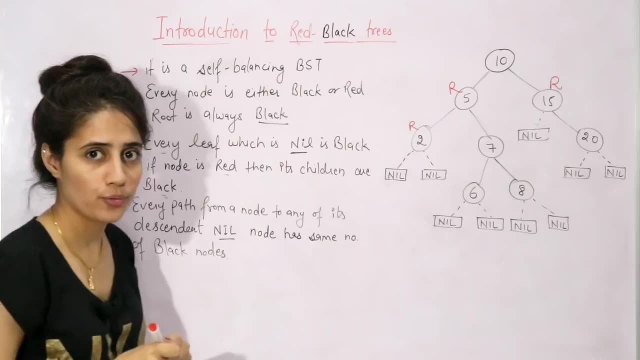 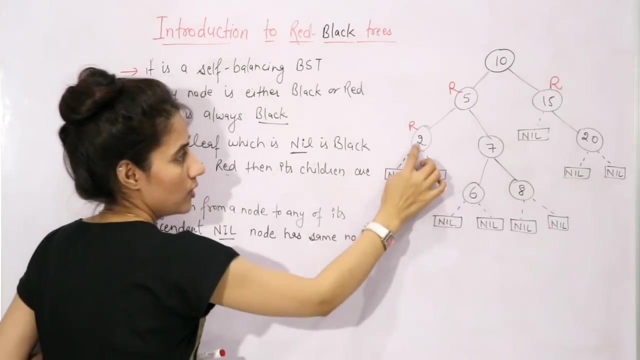 Right. So now suppose this is red and this is red, Fine, But this, if I say this is red, This is not true, Because if node is red, See, this node is red, So its children should be black. So this and this cannot be red. 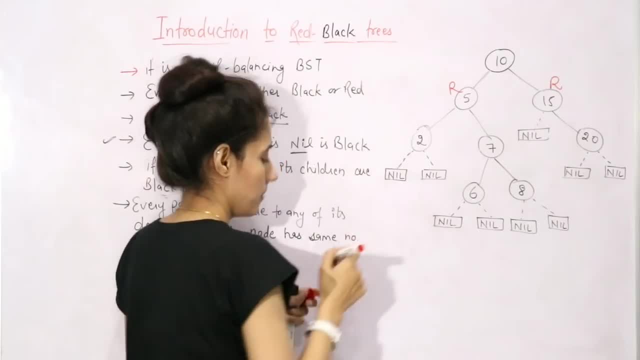 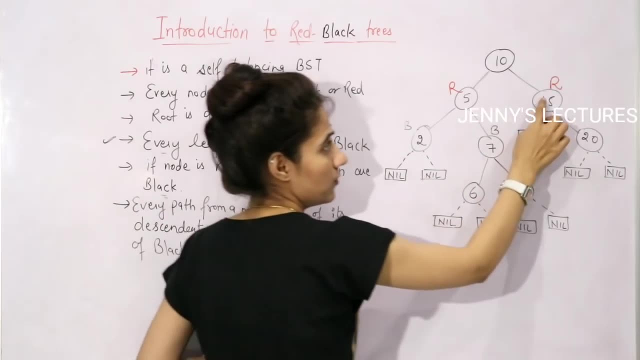 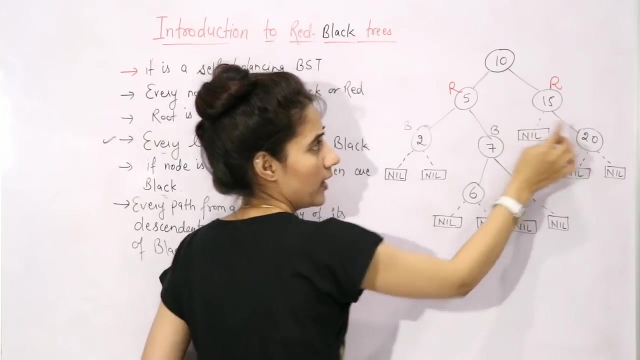 That is for sure. So this should be black And this should also be black Right. Here also you can say: if this is red, So this cannot be red Right, Because if you draw, this is red means these two are adjacent nodes. 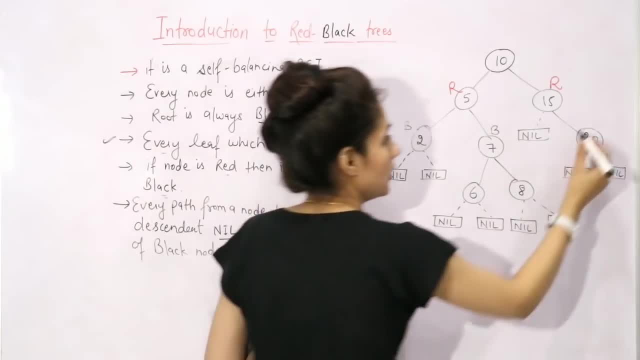 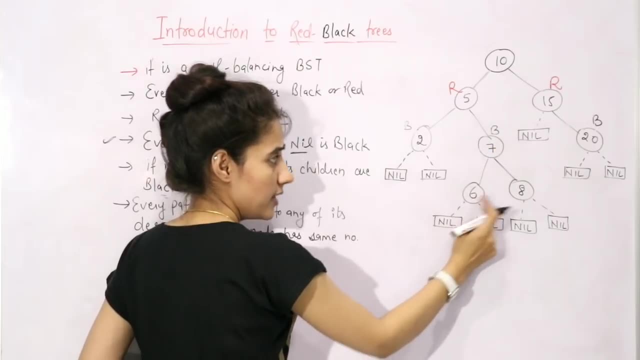 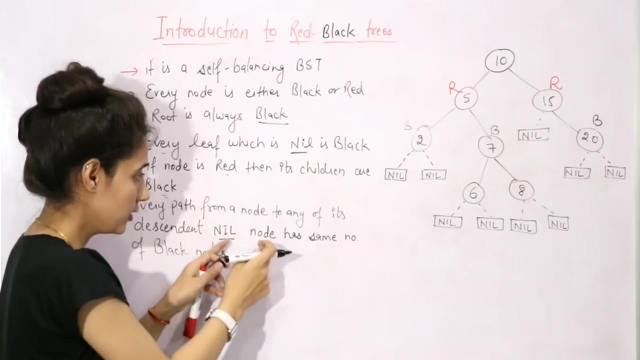 And these two are red. That is not possible, So this should be black Right Now. if this is black, Then this 6 and 8. These can be red or black According to this rule, But obviously we need to take care of this property also. 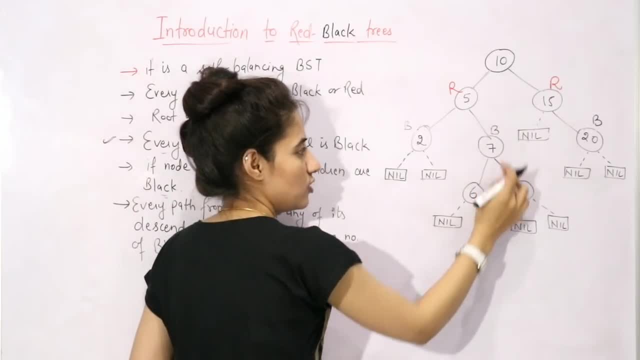 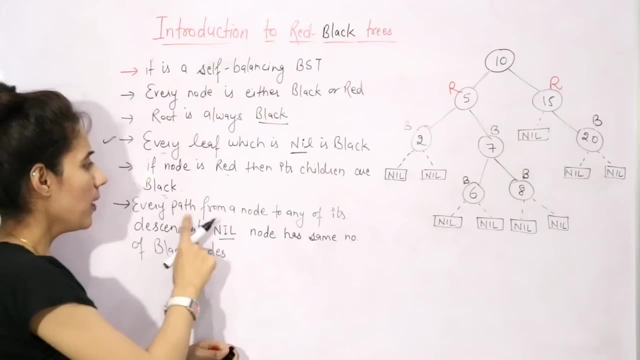 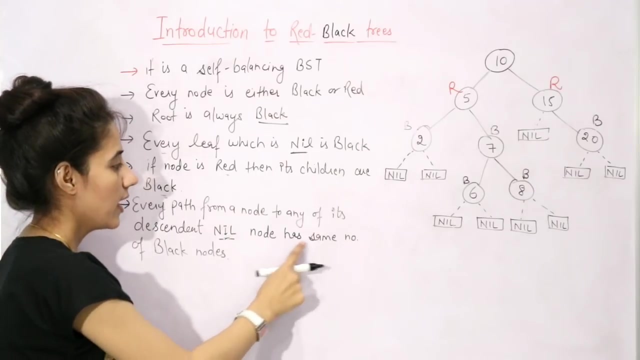 Right. Suppose, if I am taking this is black and this also, I am taking black and black. Now check the next property. See: Every path from a node to any of its descendant. nil node Has same number of black nodes. Right, Any path from any node. 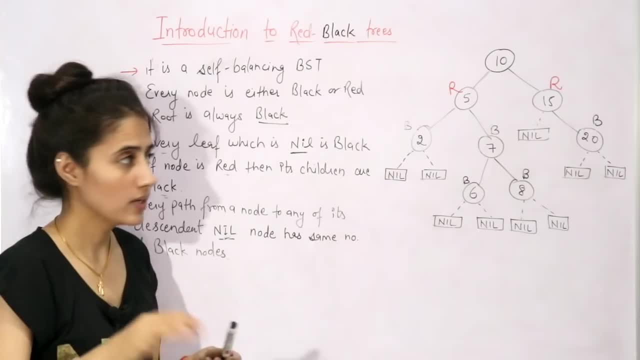 Right, Suppose I am taking first of all from the root node. From the root node, Check out the paths. One path is this one. One path is this one. One is: We can go to this nil. We can go to this nil. 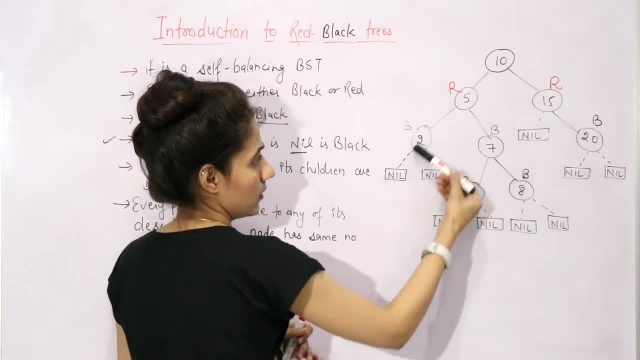 Then this, This, This, This, And this Means 1,, 2,, 3,, 4,, 5,, 6,, 7,, 8,, 9 paths can be there from the root node Right. 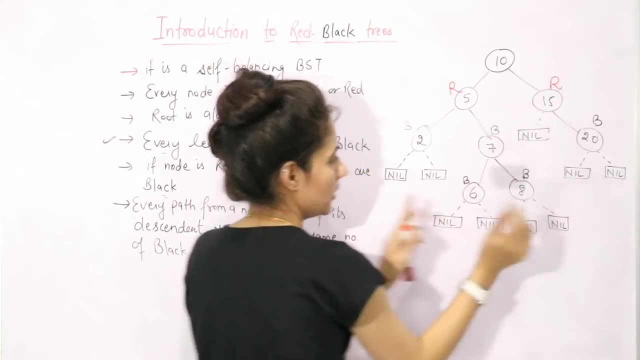 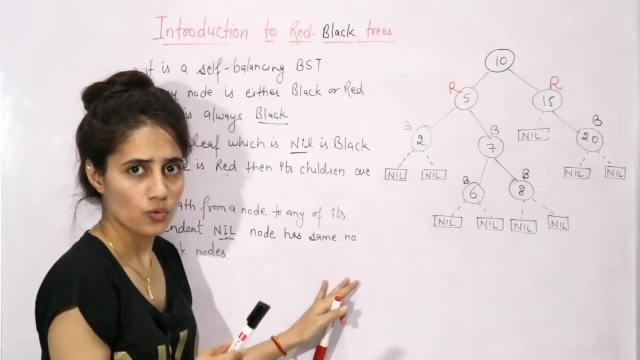 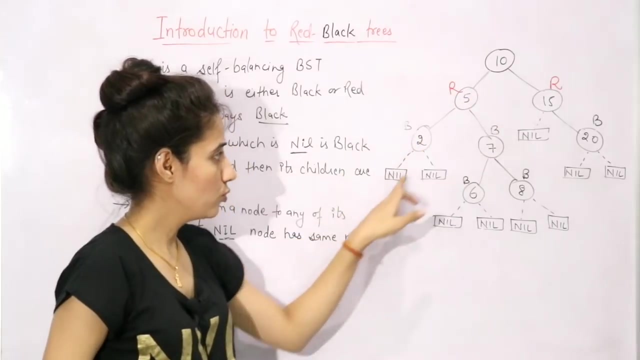 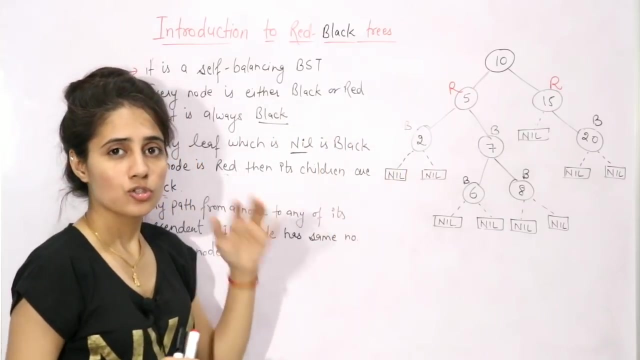 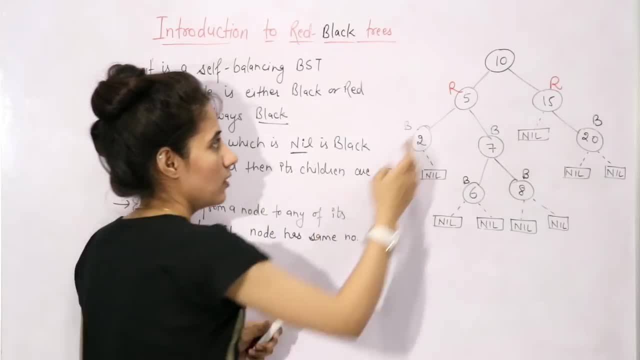 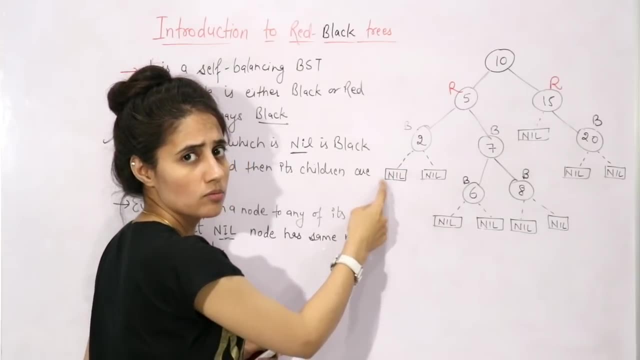 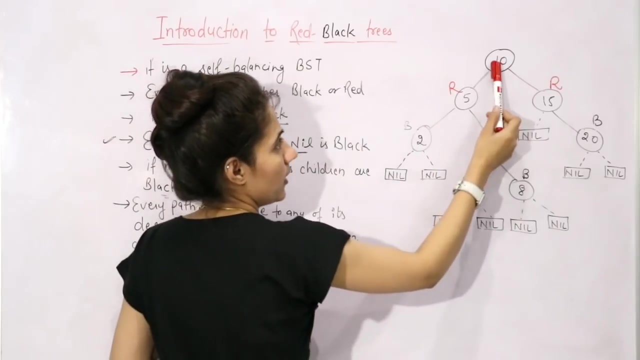 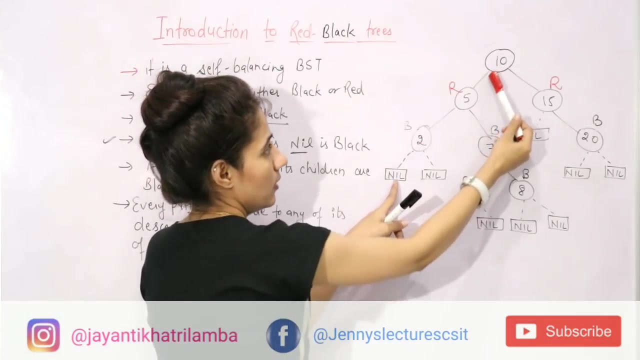 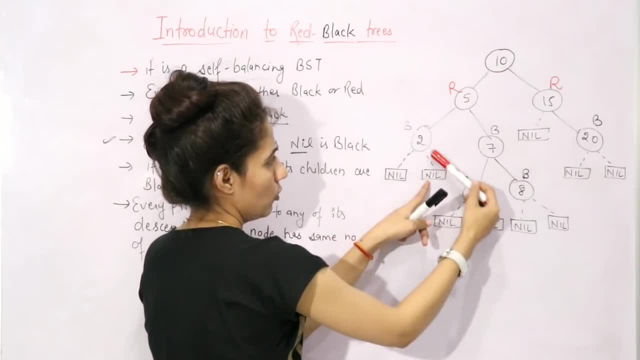 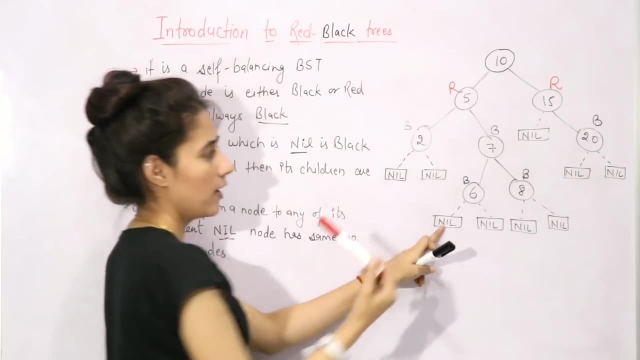 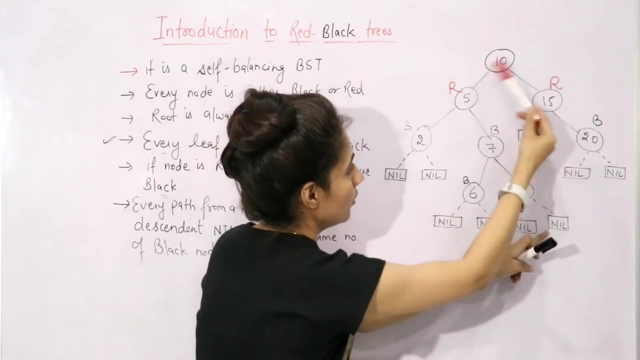 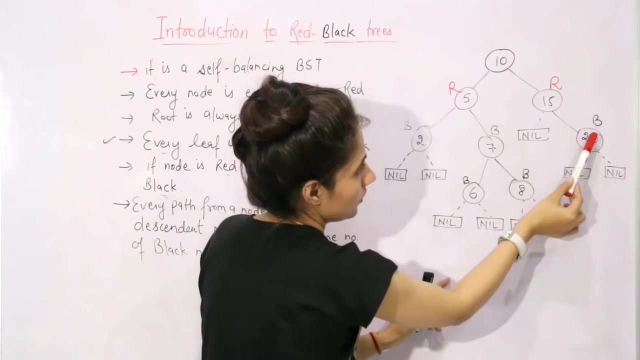 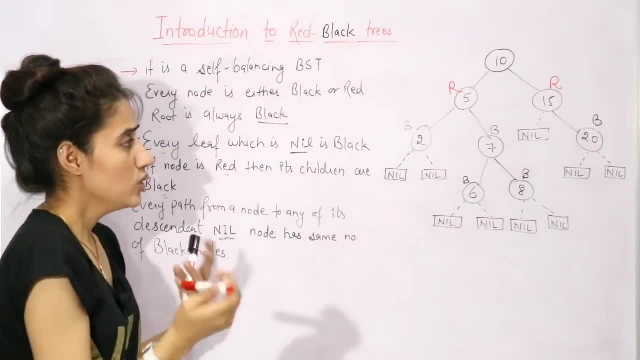 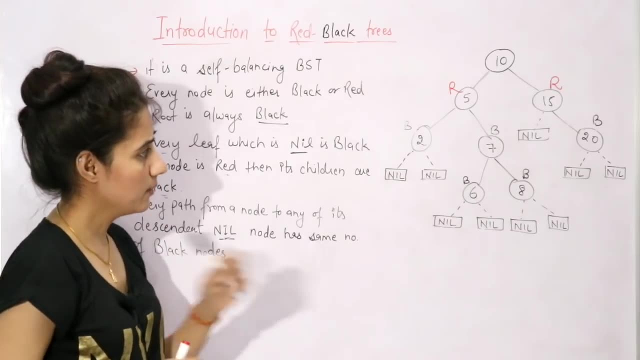 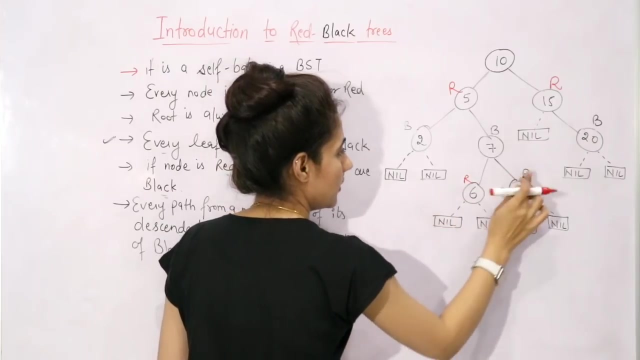 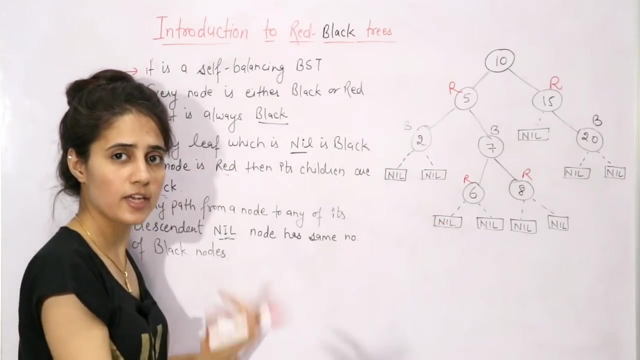 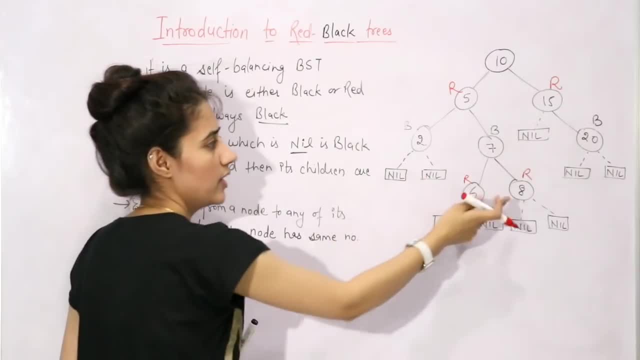 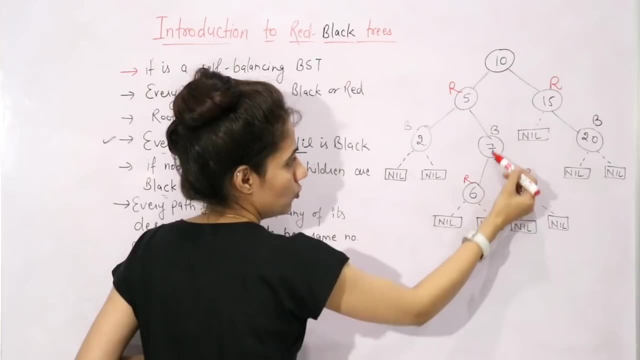 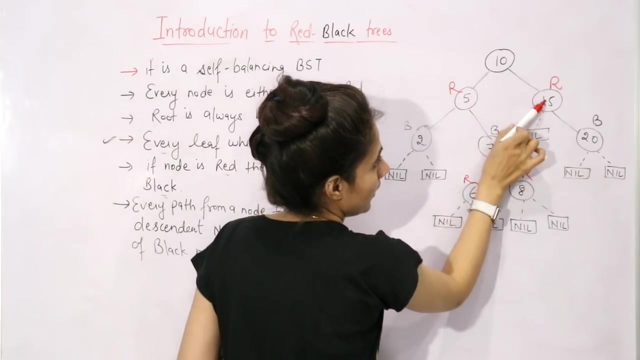 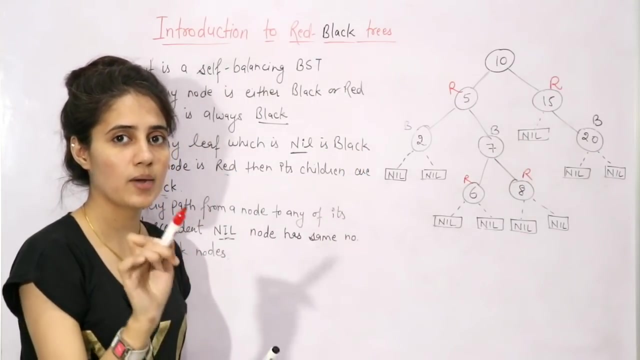 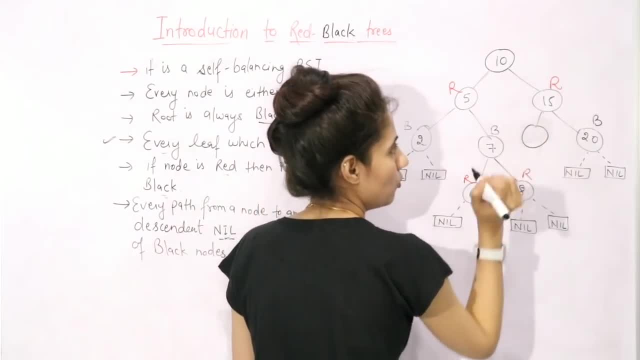 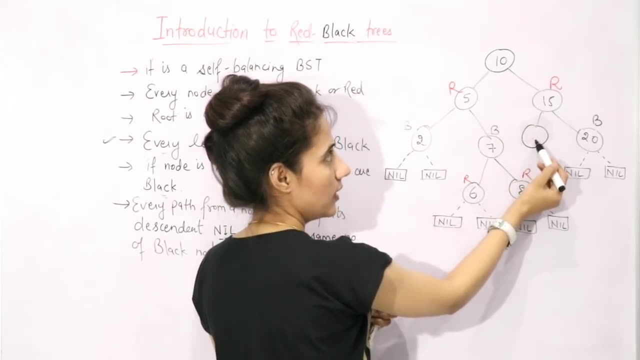 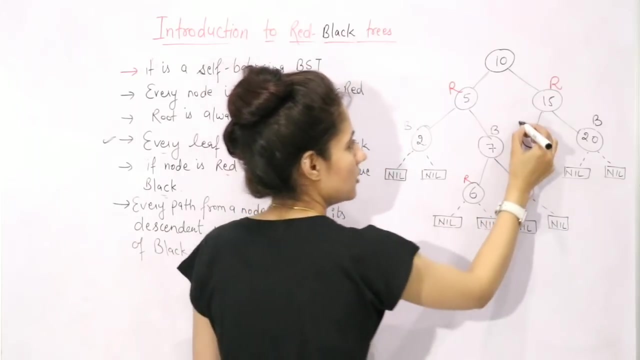 i draw here one more node and so see it is a bst. so here this should contain value less than 15, right, but it should be greater than 10. you need to take care of this thing also, right? so suppose i am taking here 12, and this is black, right. so to this also having one nil, and right also having. 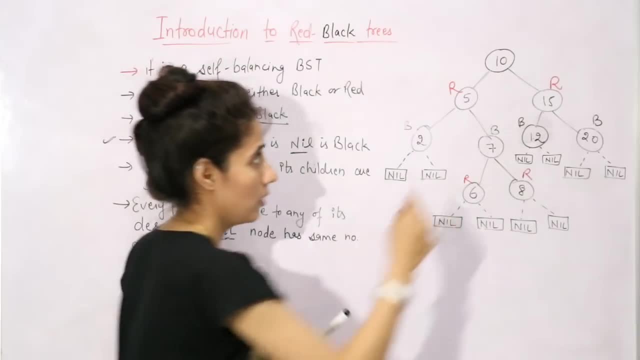 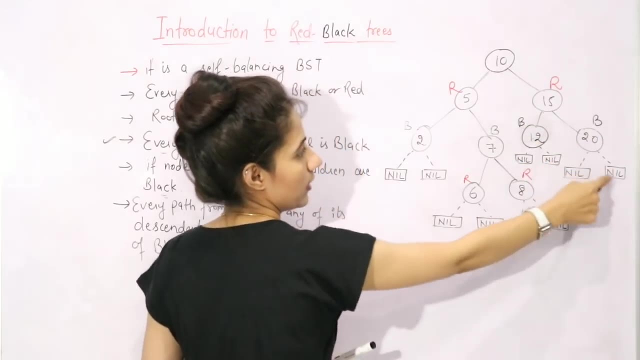 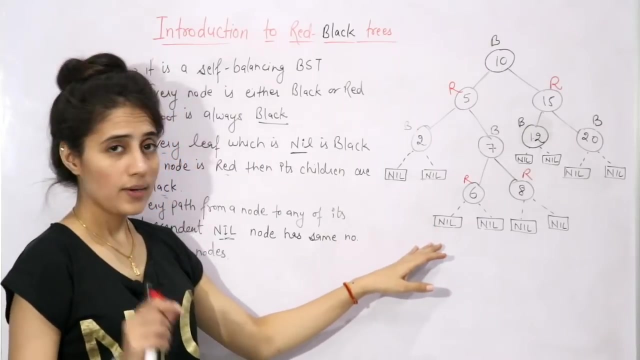 nil. now check out this path to this nil: one and two black. to this nil, we have one and two black. here also, we have two black and two black. now i guess in every path we have same number of black nodes. so now this is a red black tree. now the question may be: is every? 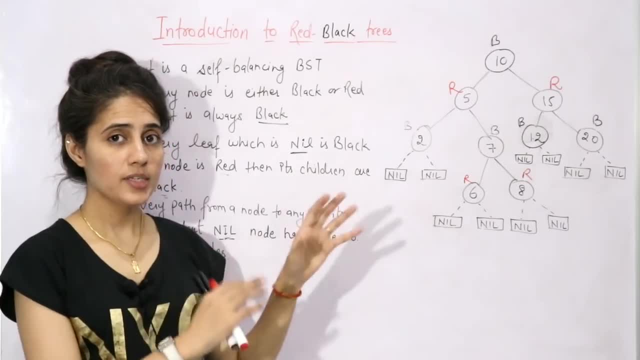 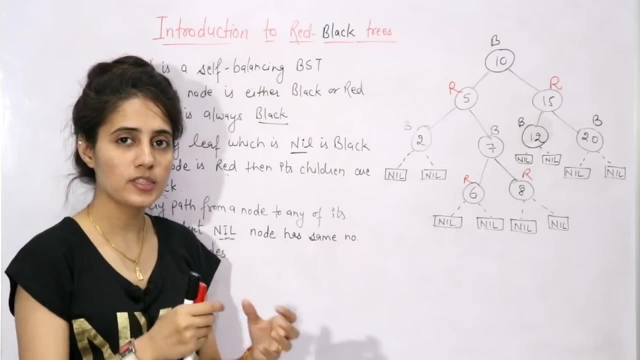 averythioisredblacknodes called something that is theärke of this avial tree can be a red black tree. see, if a tree is avial tree and you color it red and black according to the rules, then it would be a red black tree. so you can say avial trees are subset. 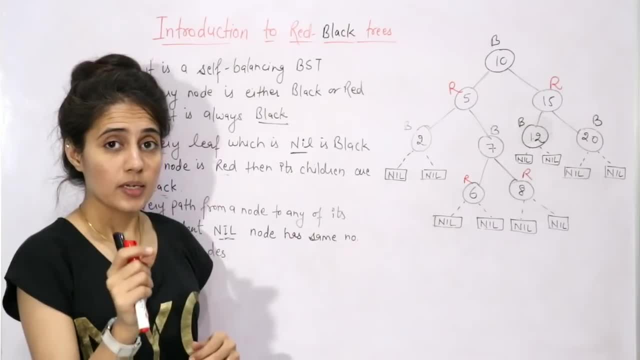 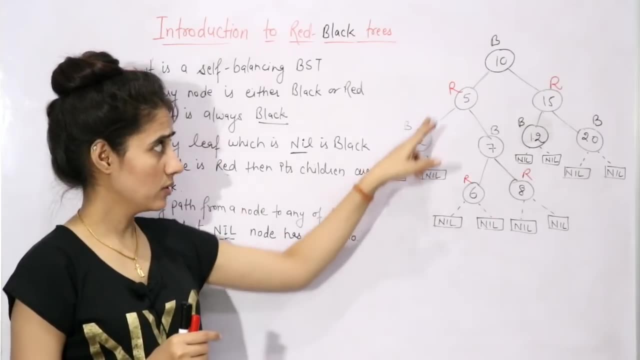 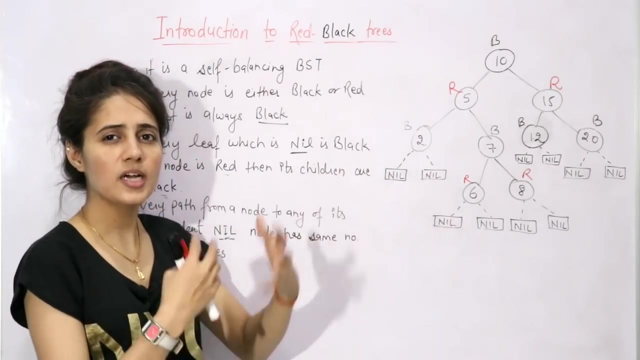 of red black trees. right, but if a tree is red black tree then it is not true that that would be avial tree, maybe if you remove the coloring. so it is not compulsory that that that tree would be avial tree, because these trees are roughly height balanced and avial tree is strictly height. 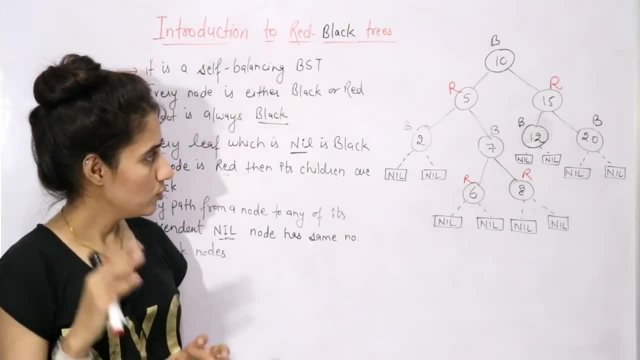 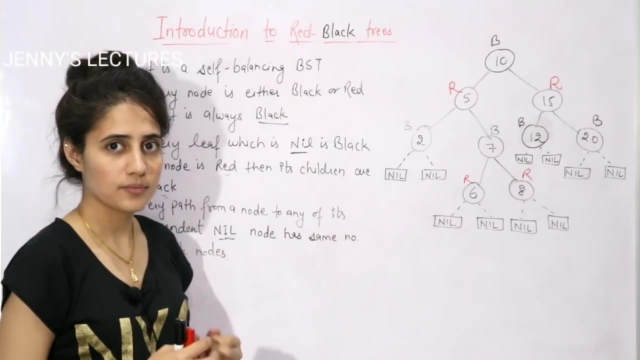 balanced tree. right now, i am going to give you some examples and we will see. are those trees red black trees or not? if not, which property they are violating? fine, so let us take these three examples. are these red black trees or not? first of all, this thing: check out this thing, see here. 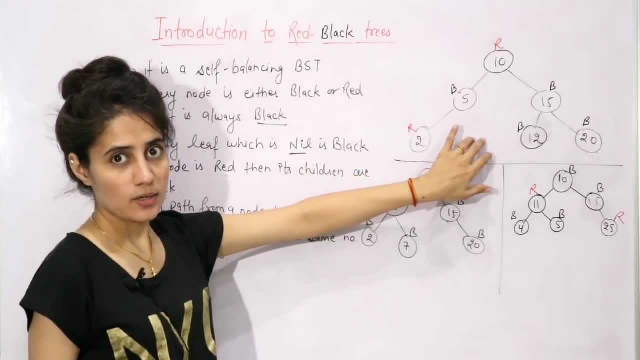 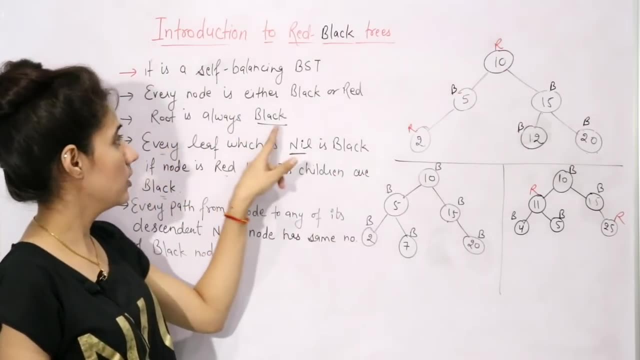 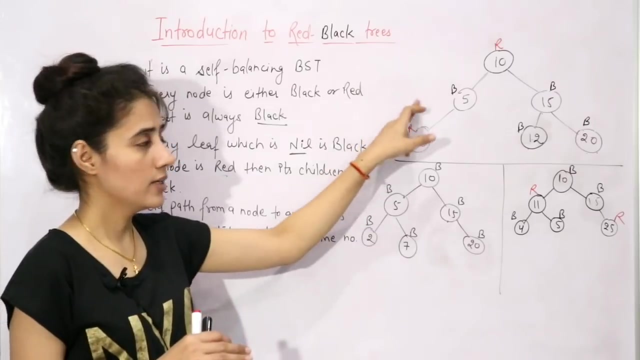 you can say first of all, it is a bst or not right, so you have to check out that condition. first thing you can say: the root is what here? red, but root should be black. so this is not a bst, no need to check out other conditions. right first is violated. it means it is not a red black tree. 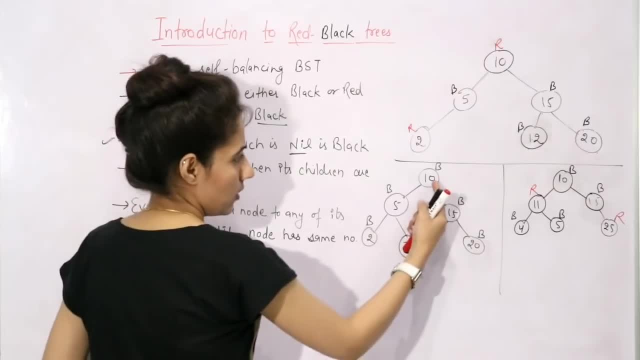 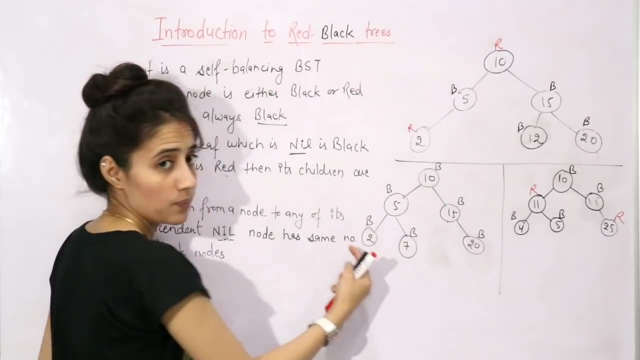 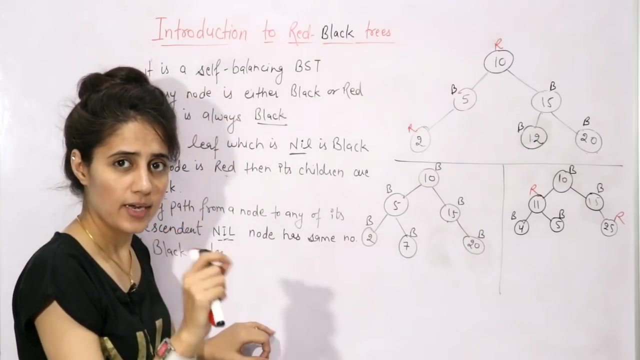 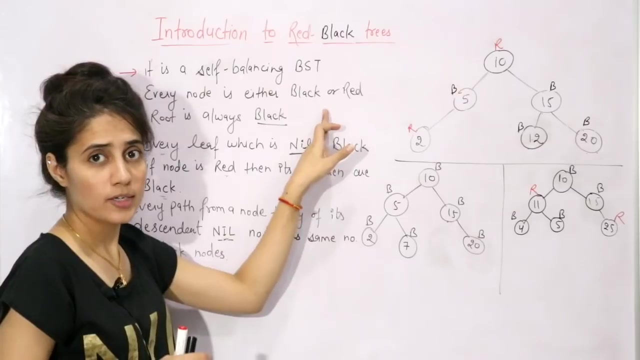 next is this one. here, see, i have, all the nodes are black, right, and obviously this is a bst because it is following a bst property right now. but this is not a red black tree. why so which property this is violating, see see, first property is what: every node is: either black or red, it is. 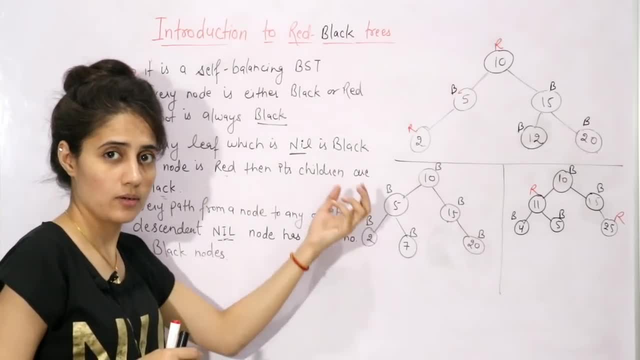 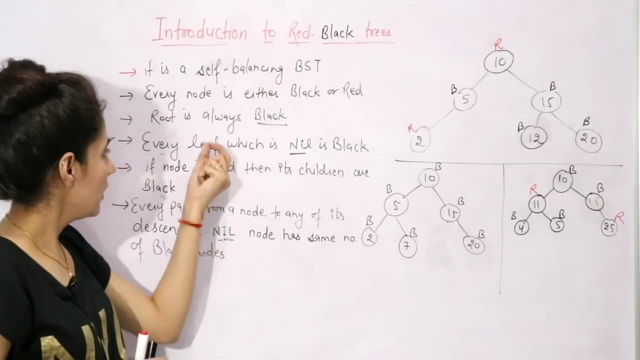 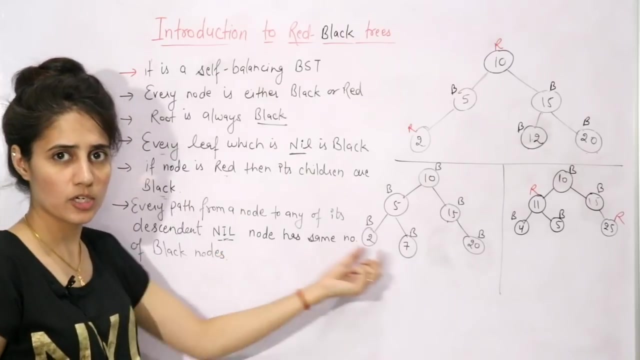 not compulsory that there should be one red or black, something like this: all may be black, because on red only we have the restriction. if the node is red, then children should be black. on the black we have don't. we don't have any restriction. we have this restriction. we will check out this thing also. now, root is black root. 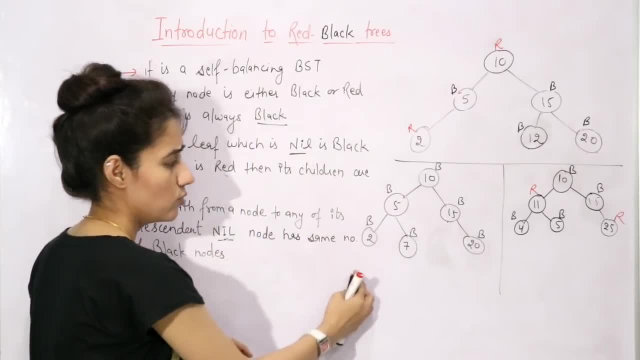 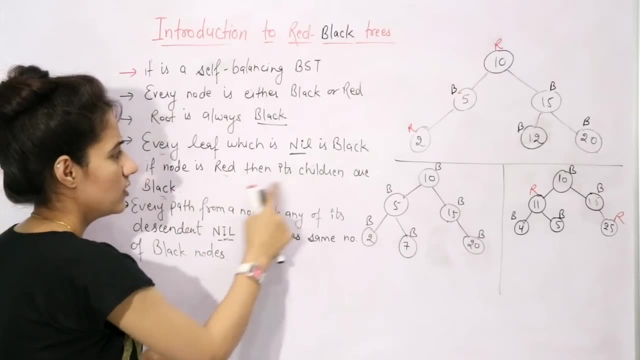 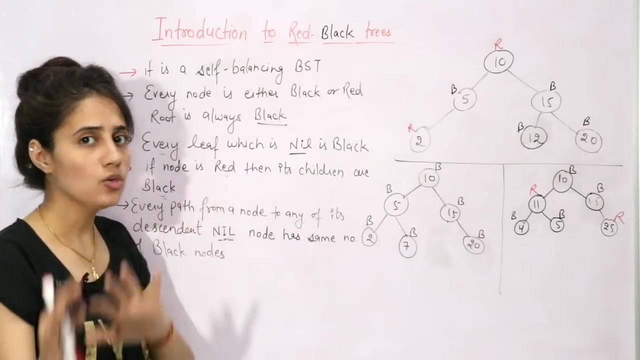 is black. every leaf which is nil is black. so obviously i'm not drawing those nil that are black. consider that thing right. if node is red, then its children are black, black. but here no red node is there. now this property see every path from any node to its descendant, null nodes or nil. 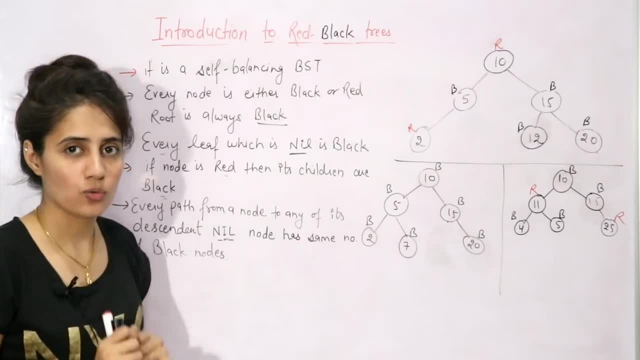 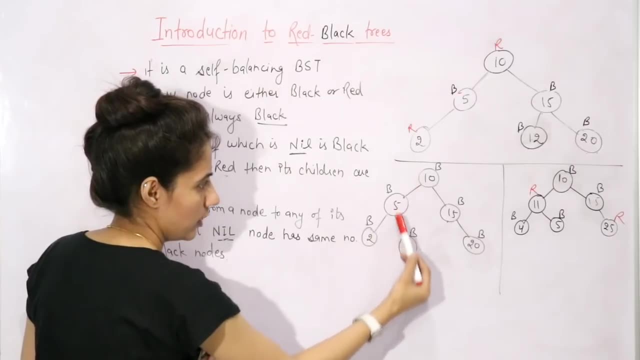 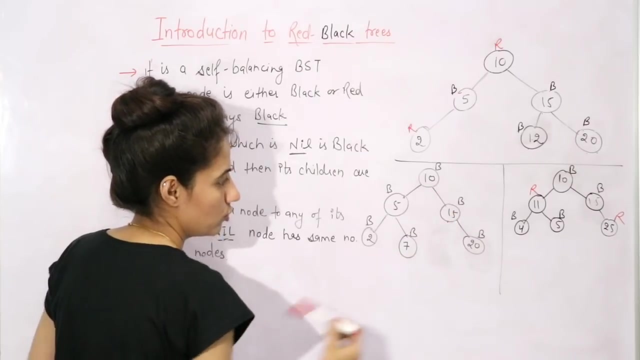 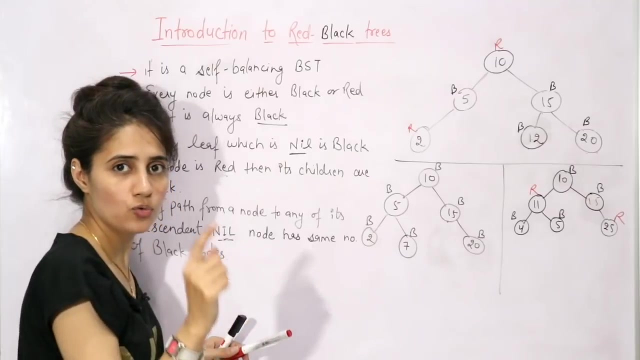 nodes must contain same same number of black nodes. now check out this path to its nil nodes: one, two, three black nodes: here also one, two, three, fine. here we have one, two, three, fine. but to this path. here also we have one nil, right. so check out through this nil one and two, we have only two black. this condition is: 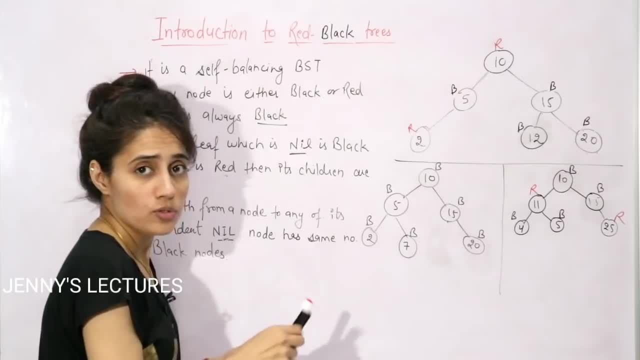 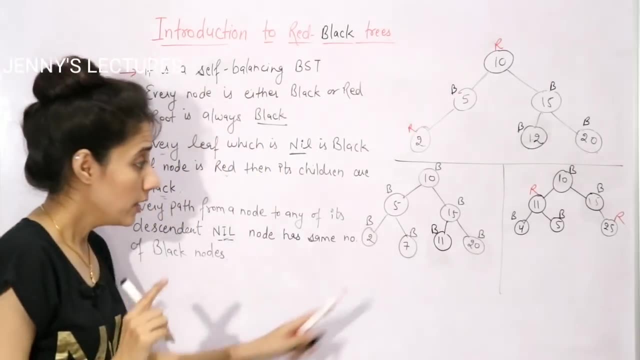 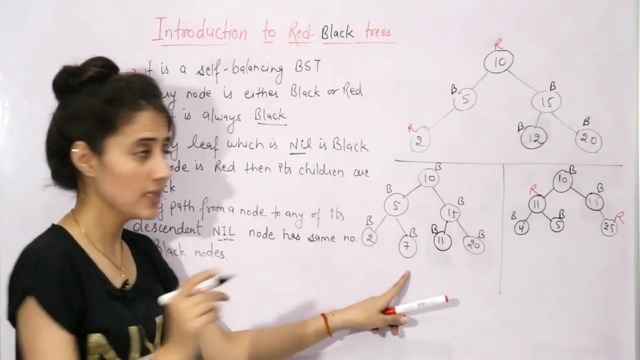 violated. so this is not a red black tree, but suppose i draw here something like this. here i have 11. this is black. now this is a red black tree. even we don't have any red color in this tree. still, this is a red black tree because it is following all the properties of red black. 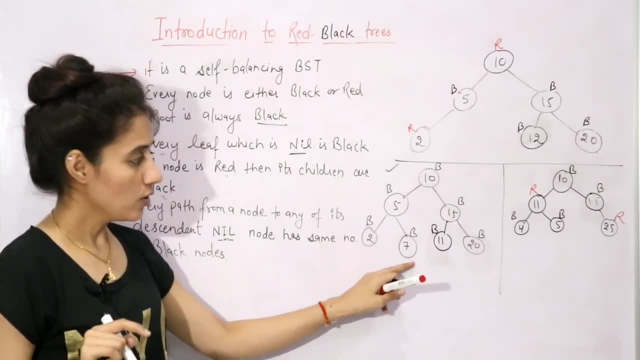 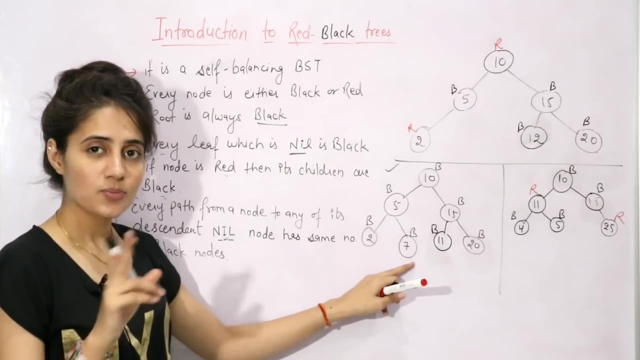 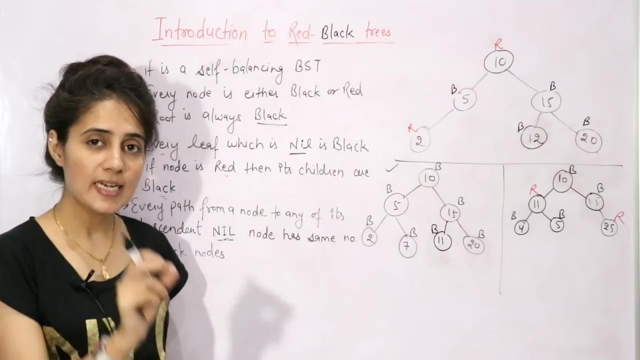 tree. so one thing you can say: it is what other than red black tree? it is what a perfect binary tree. we have already discussed binary tree and its types. you can check out that video here. what is perfect binary tree? each node is having exactly two children, and these leaf node should be. 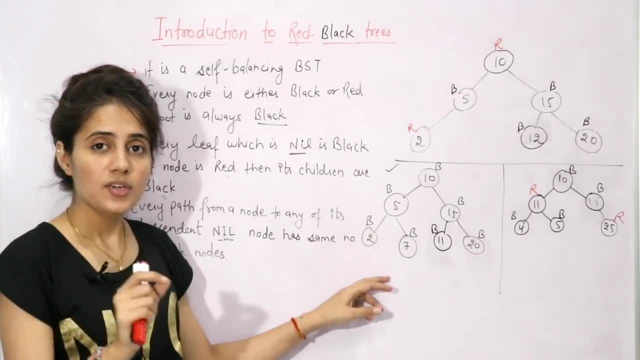 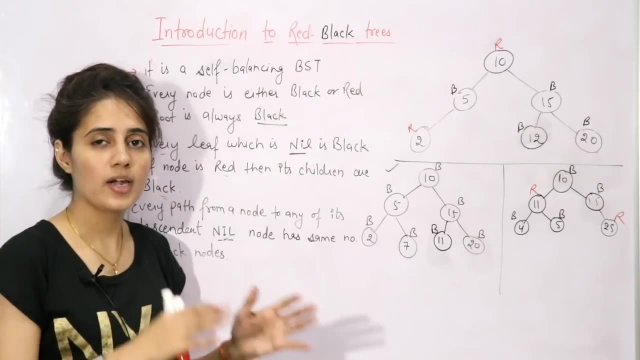 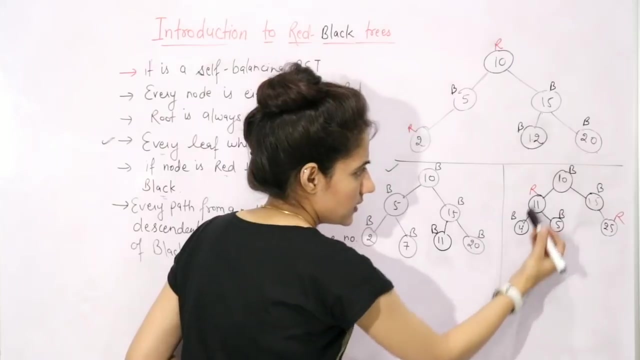 at the same level. so here you can say: every perfect binary tree that contains only black nodes is also a red black tree. so now, this is a red black tree, right, this is a red black tree. now check out this thing. is this a binary tree? binary search tree? sorry, see. 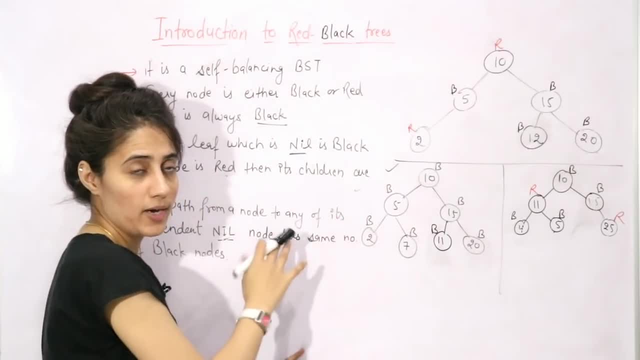 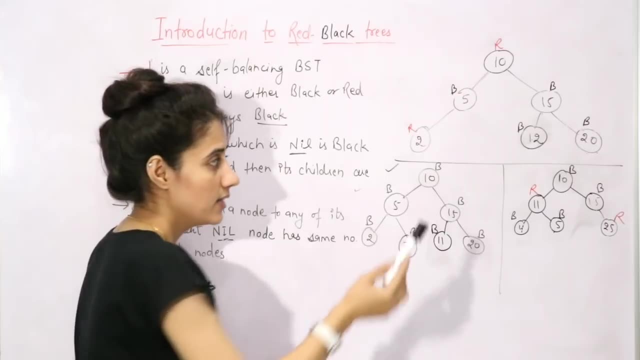 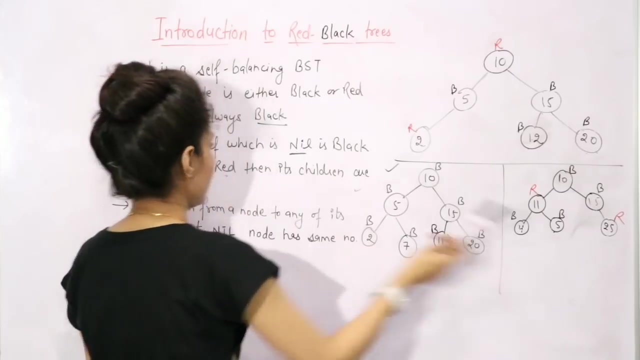 it is following all the properties of this one red black tree. if you are not checking this bst property because it is not following the binary search tree property other than that, see, root is black. root is always black. every leaf which is nil is black. obviously these are black if node is red. 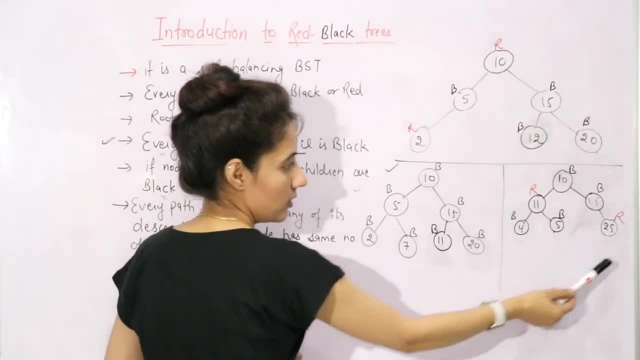 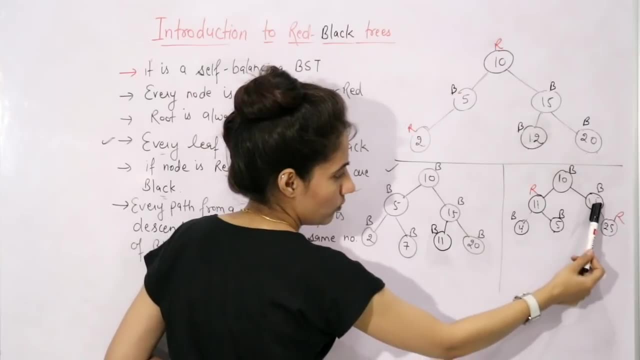 then its children are black, these are black, and its nil node that are always black. you can check out the path from here to here to black node, from here to here to black node, from here to here to black node, and here also, obviously, we are having what nil? i'm not drawing that thing, you need to. 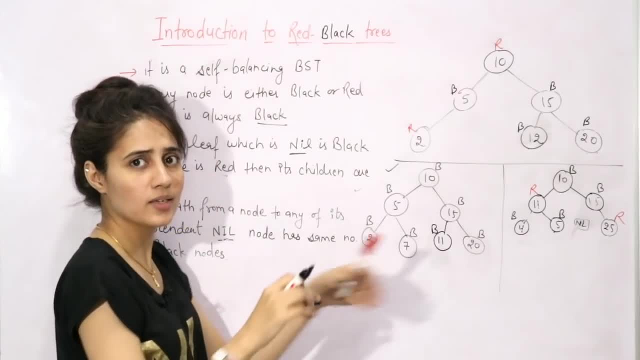 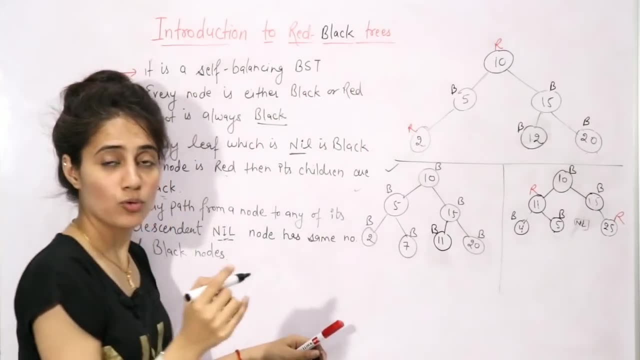 take care of this thing, because always we are going to draw the tree something like this rather than drawing the nil everywhere, right? so through this path also we have two black. so you can say this is a red black tree, but you need to check out that this is a bst or not. this is not a binary. 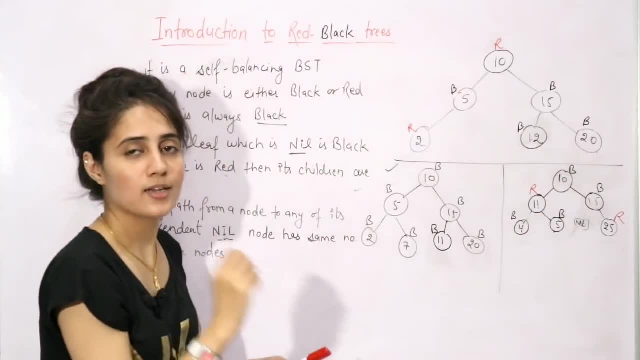 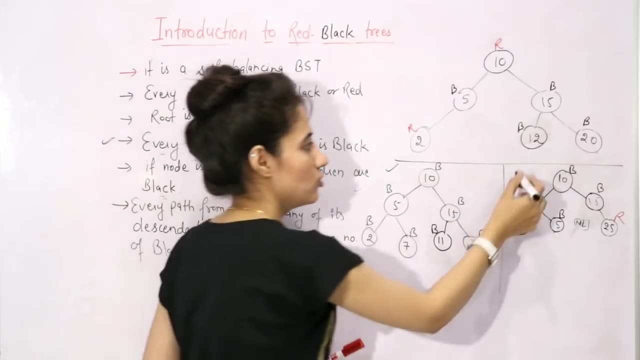 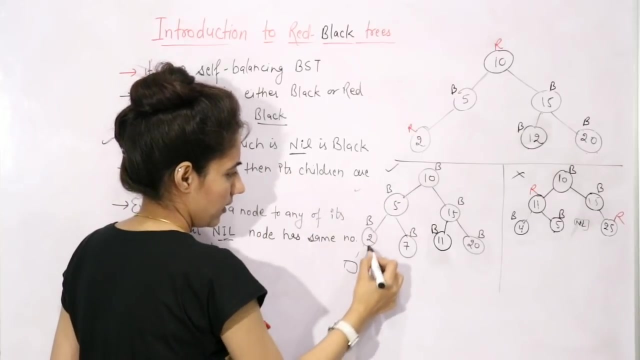 search tree: see: to the left of 10, we have 11. that is not possible. to the left of 10 in the left subtree, we should have you use less than 10. so this is not a red black tree, right? see? rather than writing all here, nil for. 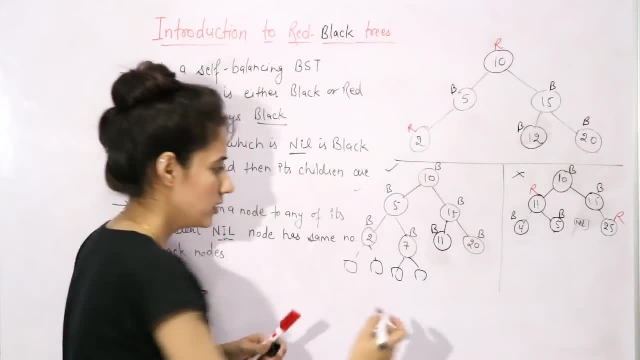 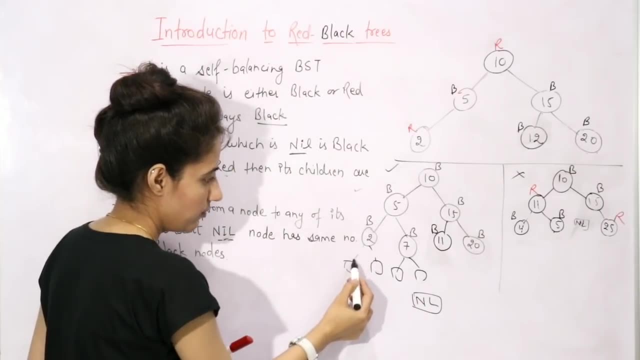 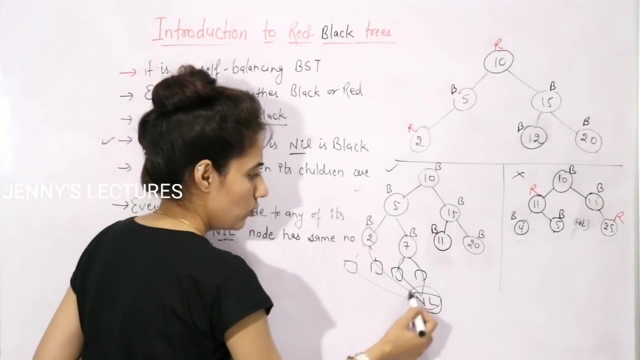 every node, for every leaf node, what you can say. one node can be nil, that can be sentinel node and you can connect- see the left pointer of this to this, the right pointer of this to this left pointer of this to this nil, right pointer to this nil. so you need only one sentinel nil node. 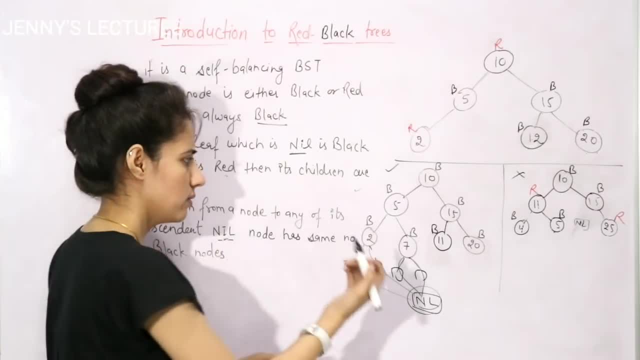 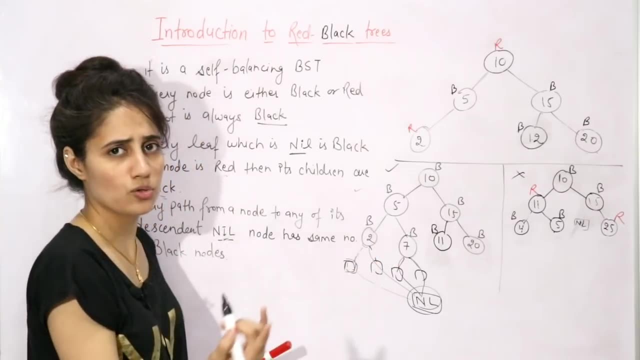 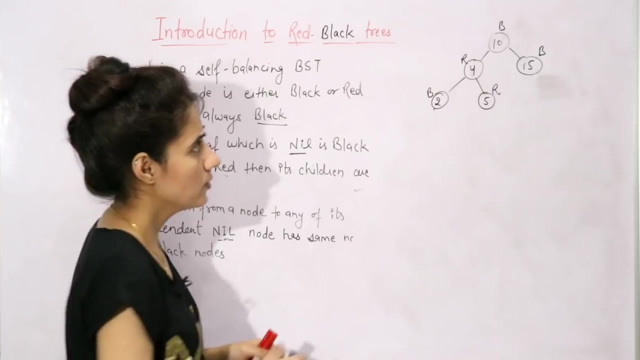 that also. you can implement something like this, or rather than this, you can consider: for each leaf node, for each these leaf node, one nil node. that is also fine. right now we will take some other examples. now check out for this tree: is this a red black tree? it is a bst. yes, root is black, yes. 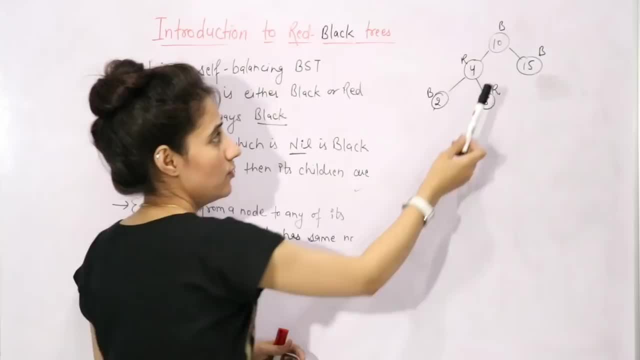 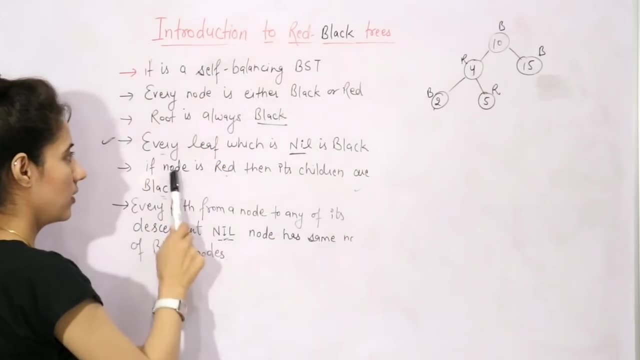 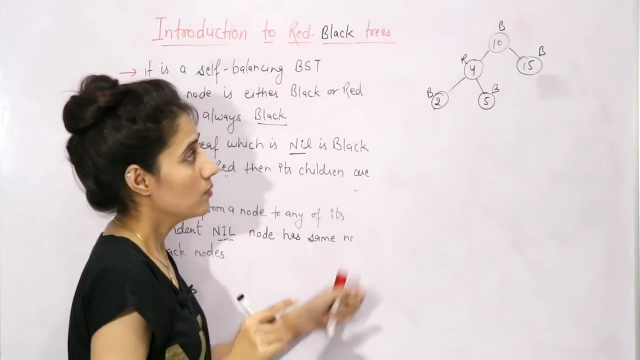 but see, this is red. this is also red. but if a node is red, then its children should be black. so so this is violating this property, the this one, right? if i write here black, then then is it is a red black tree, right? this property is also followed. now check out this one, check out the path from. 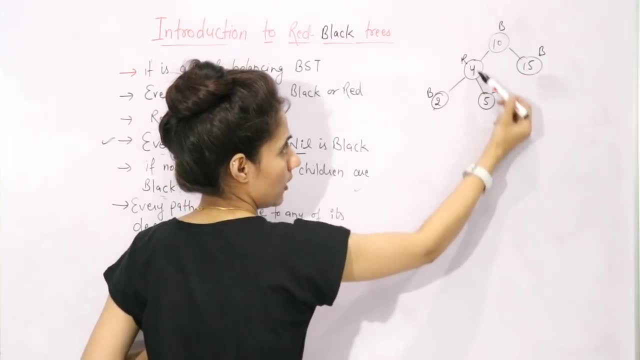 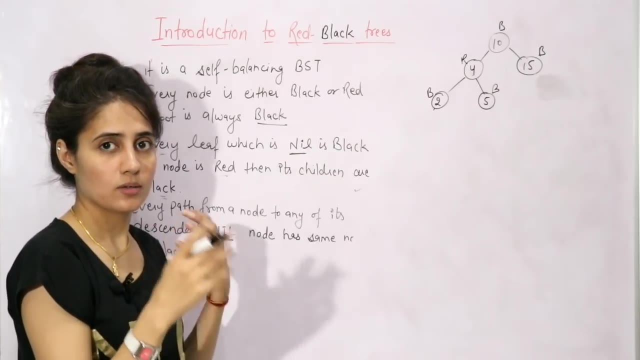 here to here we have one to two black nodes. from here to here also two black nodes. from here to here we have also one to two black nodes. so every path is having same number of you can say that black nodes. see, this condition you can check out from any node. see, suppose i am taking this node. 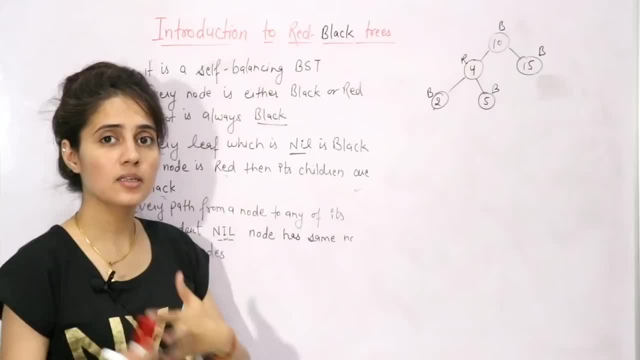 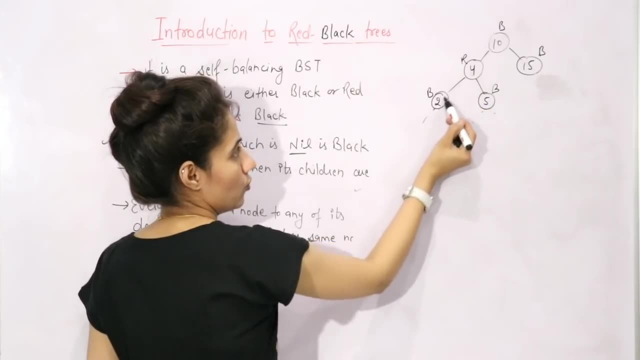 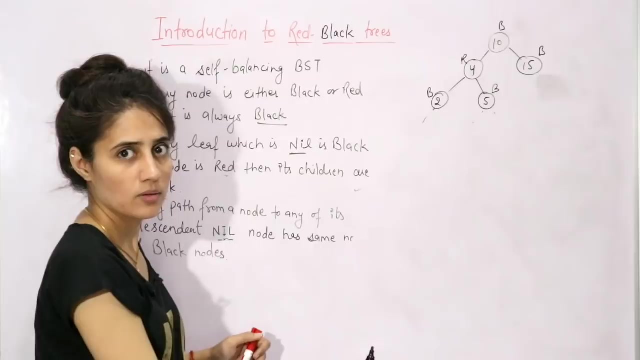 from this node check out the path to its descendant nil nodes. so here we have this path, because here we have two nil nodes, here we have two nil nodes, so one to this node, that is one black node from here to here also, one from here to here, one from here to here, one right. so this. 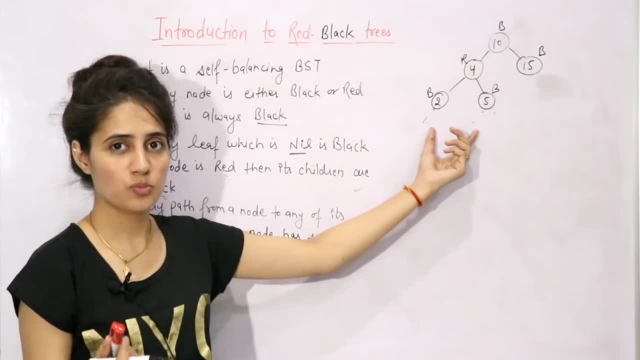 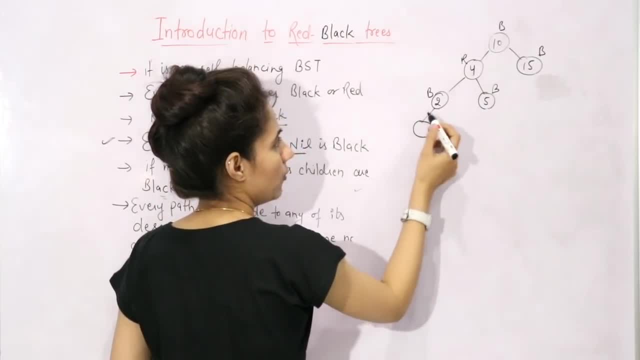 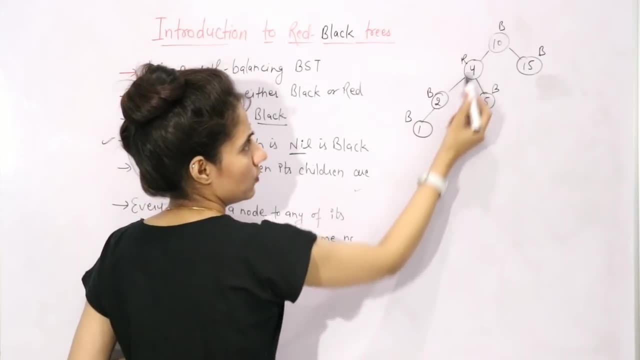 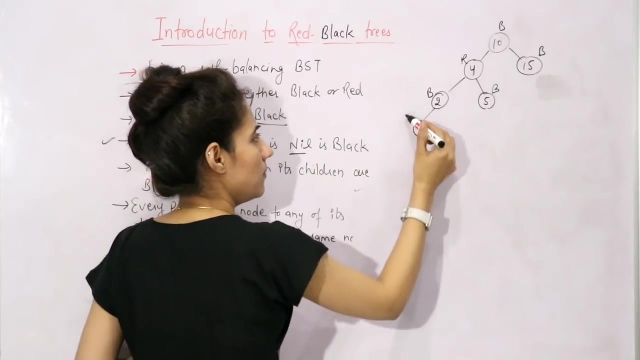 if i draw here one more node, and which is what? suppose black, and this is one. now, this is not a red black tree, because in this path we have one, two, three black nodes and here we have two. so this is violating this condition. this last condition, suppose i am. 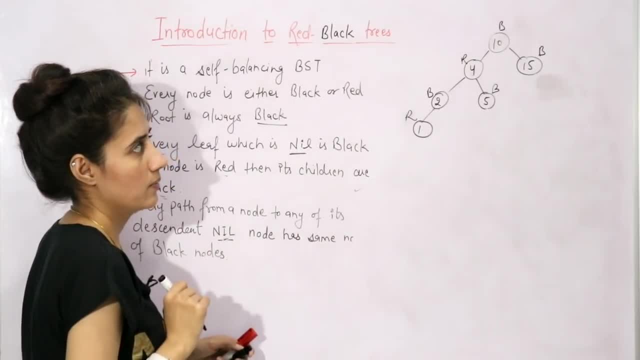 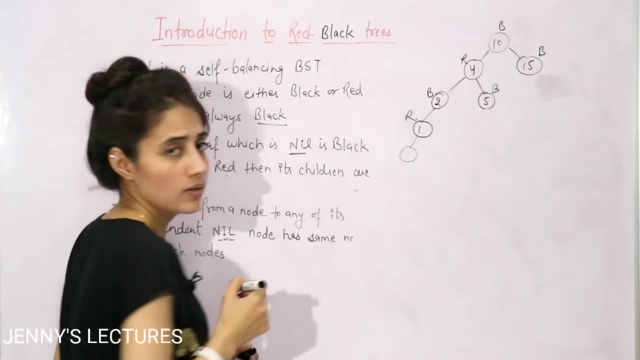 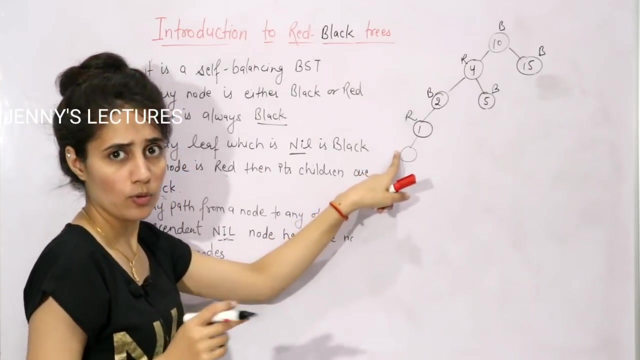 changing the color to red. now this is a red black tree, right. so now, can you, can you extend this further? can you here draw one more node? see, we cannot draw red, because two adjacent red are not possible. if you do the coloring black right, suppose 0, i am taking, so in. 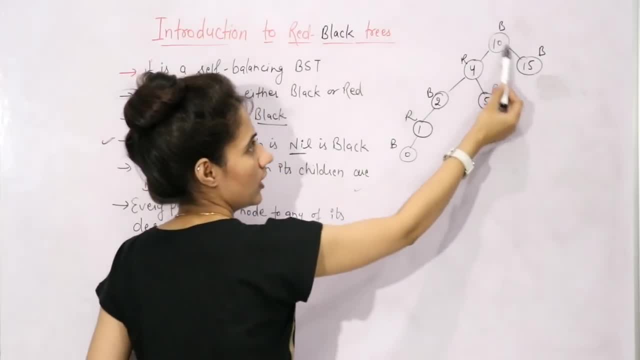 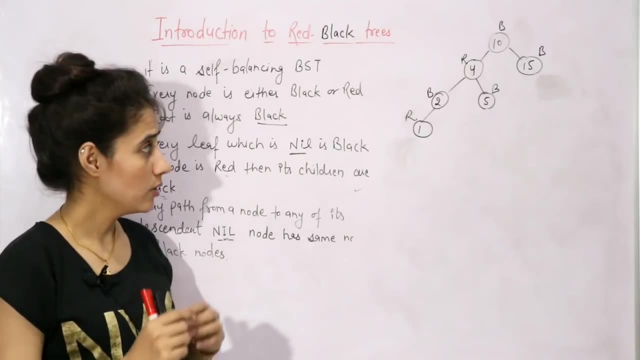 this node b, 1, 2 and 3, 3 black nodes, but here we have only two black nodes, so this is not possible, right? so now here one more point about red black tree is what we are drawing that point from this property? only because this, because of this property, we cannot add here one more node. 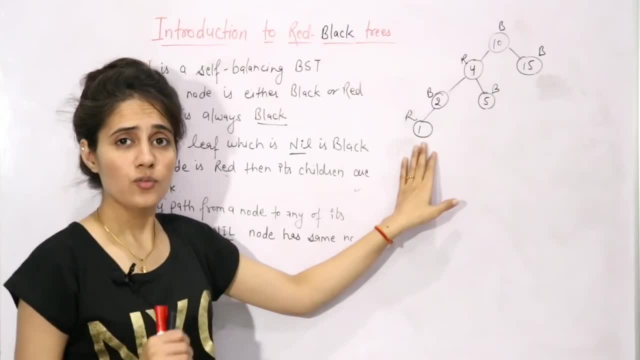 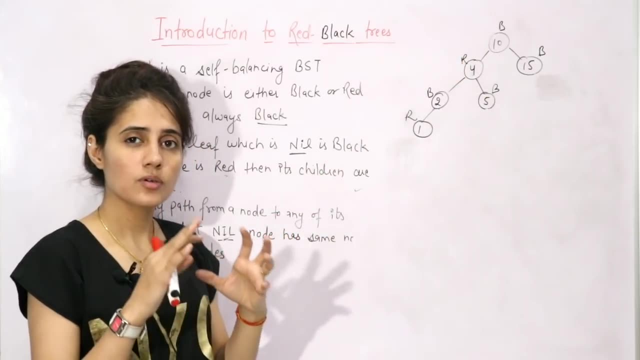 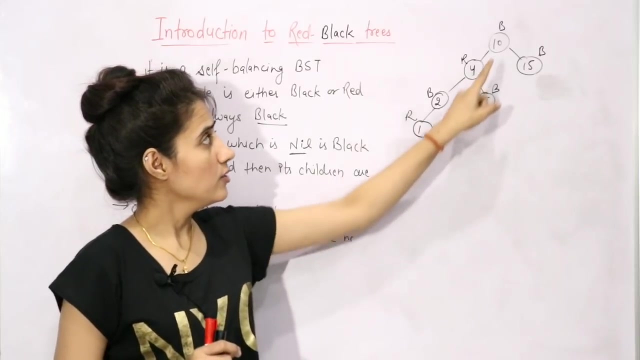 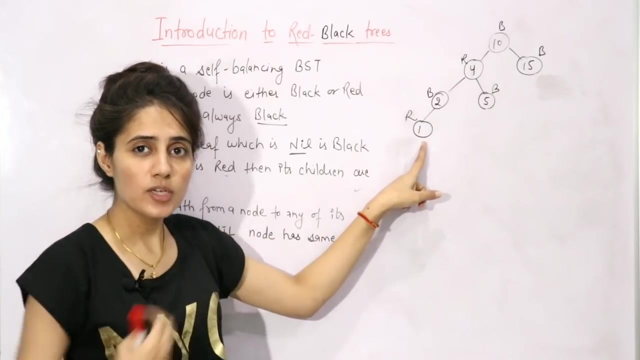 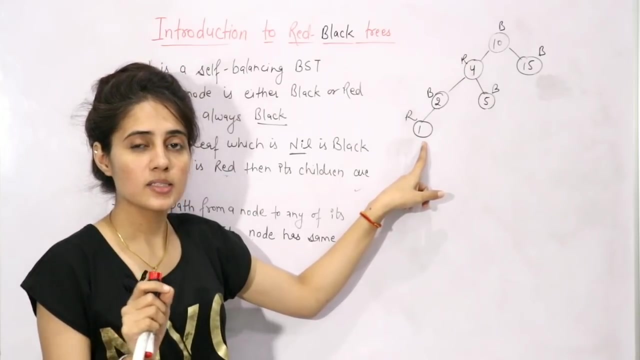 neither red nor black right. so here you can say: the longest path from the root is no more than twice the length of the shortest path. or you can say: see, the path from root to its farthest leaf node- farthest means to its extreme leaf node right- is no more than twice as long as the path from root to its nearest leaf node. now, 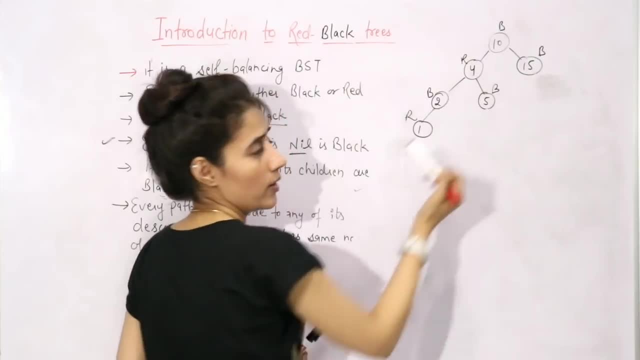 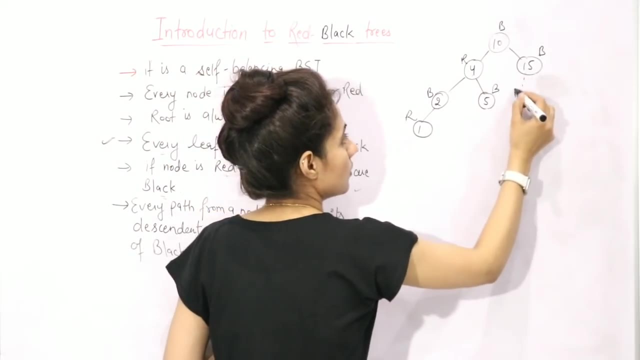 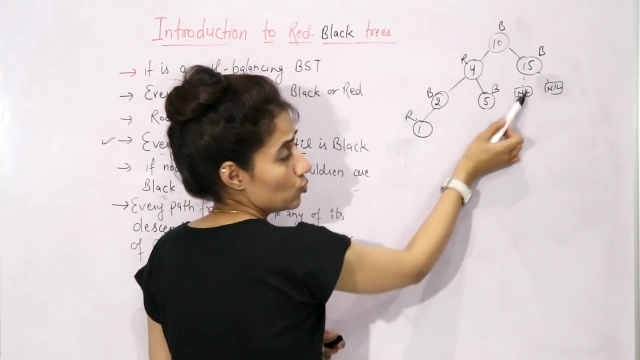 see the nearest leaf node of this root. is this one, right? if you don't consider this, then here you can say: these are leaf node. that is nil and nil, right? so nearest are these one, these two? so this is the nearest leaf node and this is the nearest leaf node, and this is the nearest leaf node. 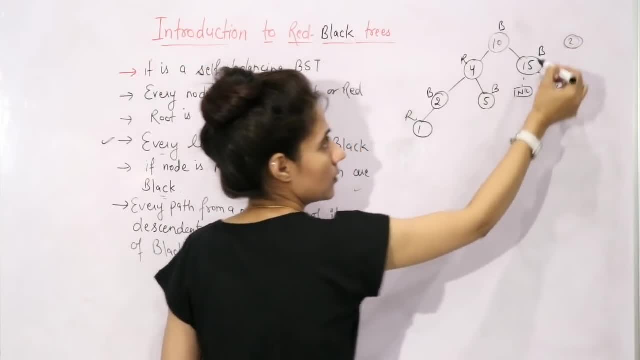 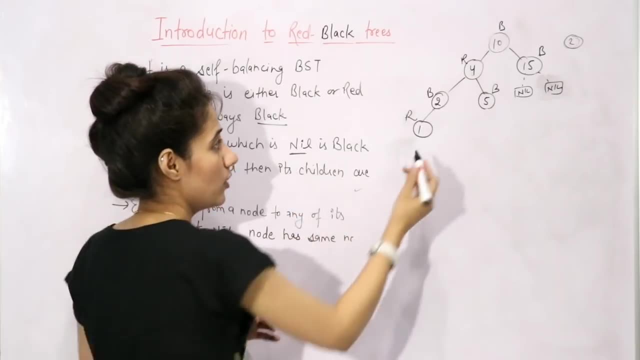 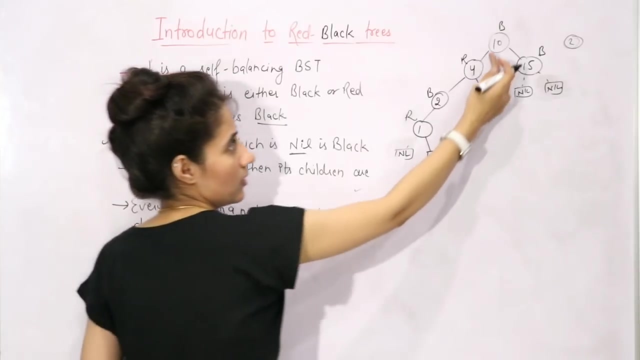 of the path is 2 right now, the, the extreme uh leaf node, or the farthest leaf node is this one. or you can say here we have nil and nill these ones right. or you can say the extreme at the maximum distance from the root, these are the nodes. 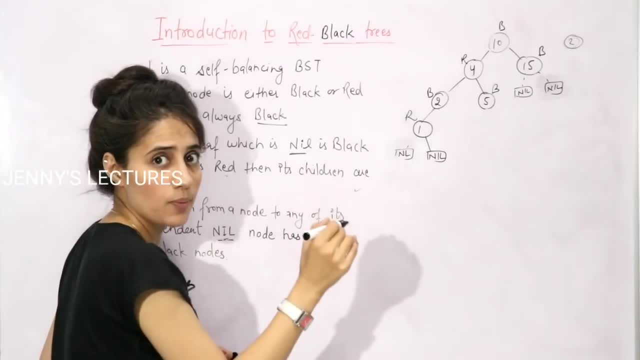 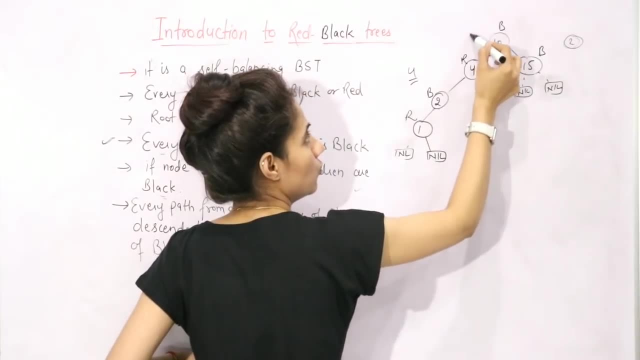 so check out the path here. what is the path? having 4, this to this, then this to this, that is one, so 4.. 4 it means 2 into 2, that is 4. it cannot be more than 4. so you can say it cannot be more than. 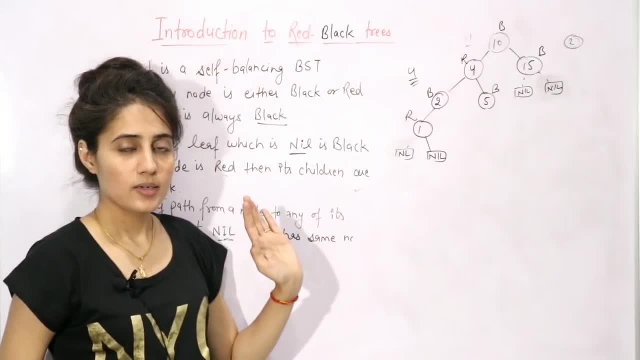 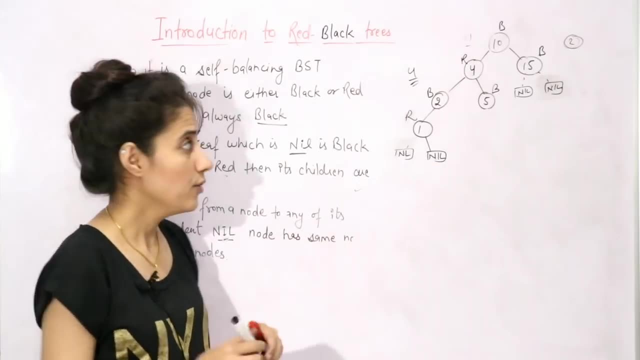 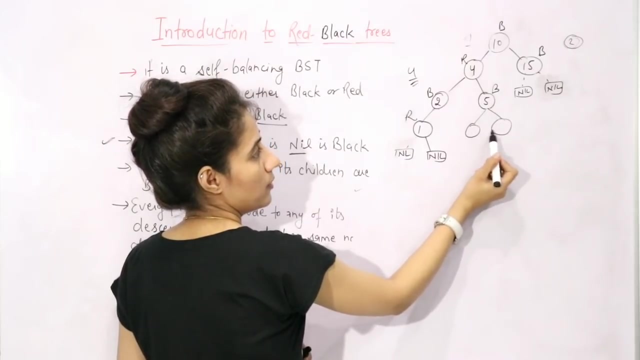 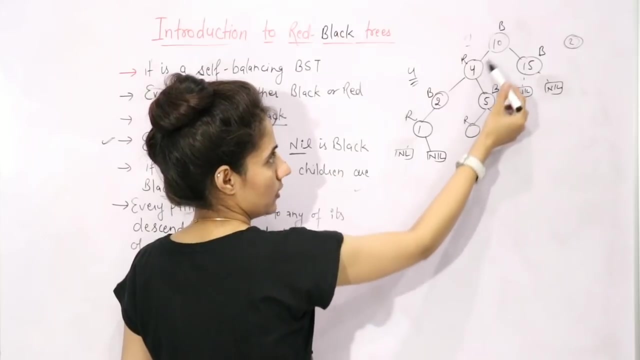 twice, then this path, right, that is one more. you can say that point about red black trees. i hope you are getting this property. see, here, we can add some node here, right, so these nodes can be what red, these cannot be black, because if these nodes are black, then 1, 2 and 3 in this path. 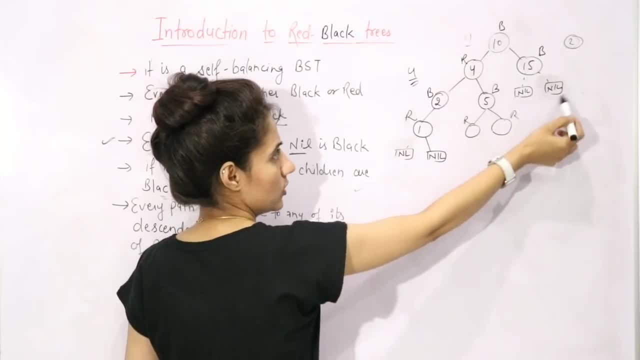 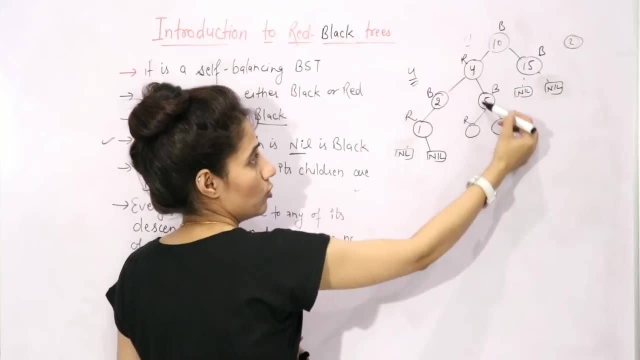 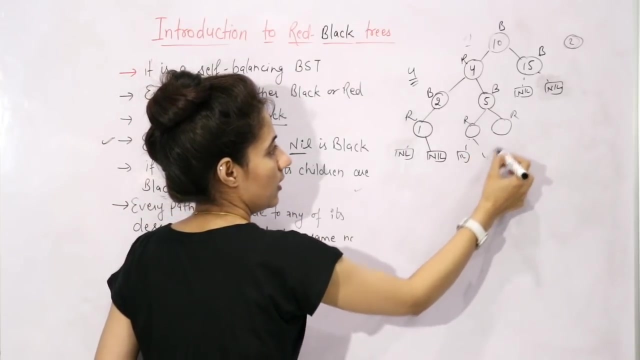 three black nodes are there and here we have only two black nodes. obviously we are not considering these nil nodes, right? so here you can say red and red, that is possible, right, but this is also what this path is also having. what value? 4: here we can say nil, nil, nil, but here further we cannot. 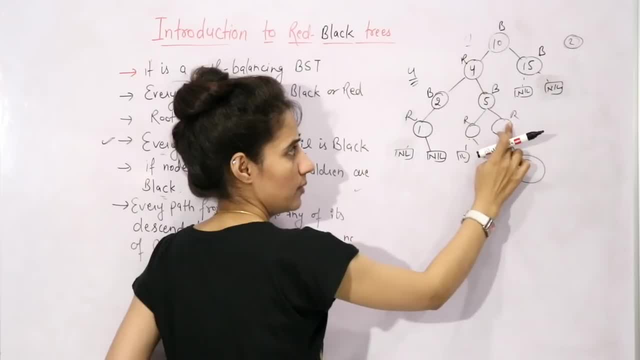 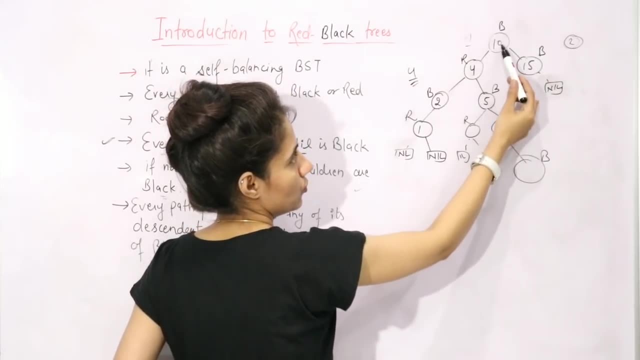 insert nil, nil, but here further we cannot insert nil, nil, but here further we cannot insert nil, nil. any node, either red or black, red, we cannot insert because it is red, red, this condition would be violated. we cannot insert black, because if you insert black, then here one, two, one, two and 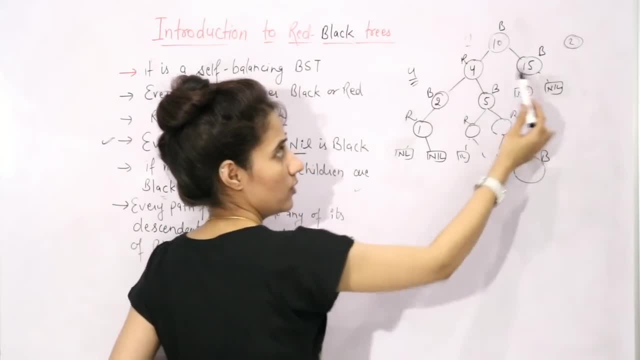 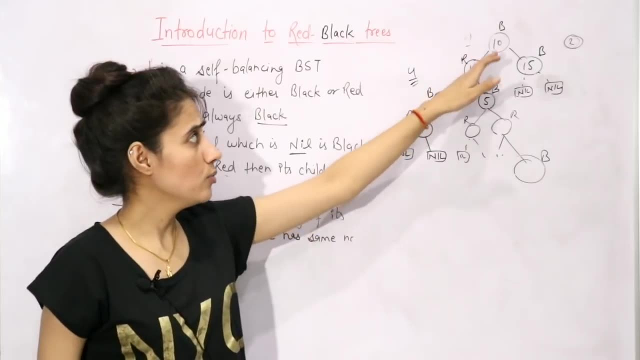 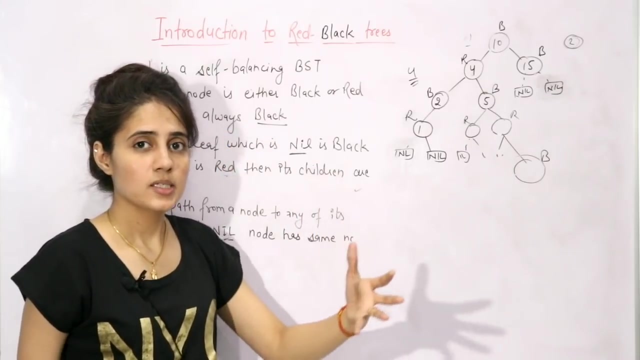 three, three node would be there, black node would be there to this path, and here we have only two nodes. so that is one more point, and that point has been, you know, driven from this point only, the longest path from root to its leaf node cannot be, you know, more than twice the length. 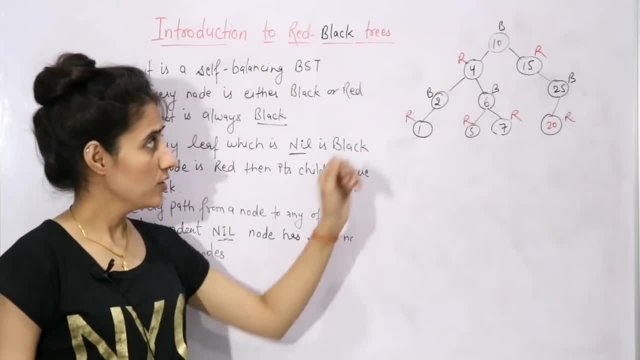 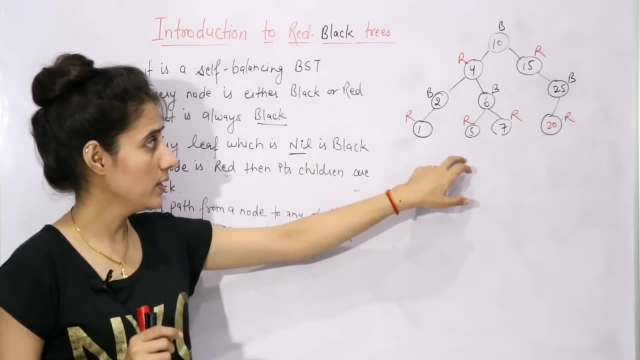 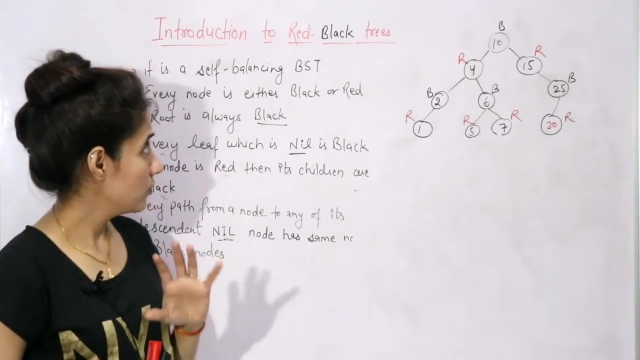 of the shortest path. so now this is question for you. you need to tell me: is this a red black tree or not? if not, then which property this tree is violating. you can write down your answer in the comment box, right? so this is now just fine, i guess, for the introduction part of red black trees. 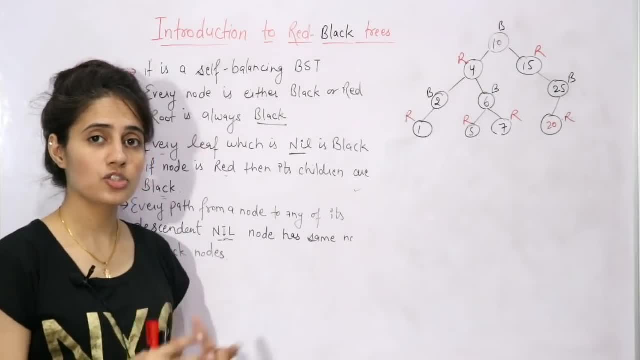 in the next video we will discuss the how to perform insertion in red black trees. right, so i'll see you in the next video. till then, bye, bye, take care. 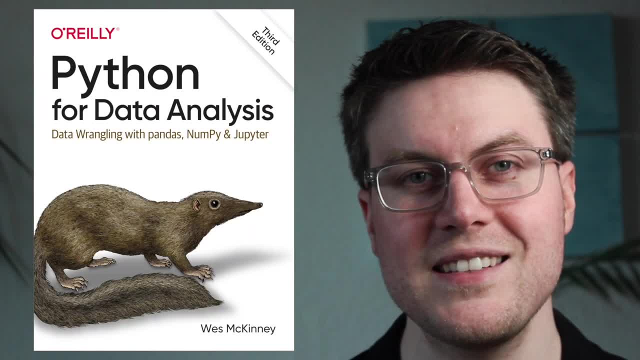 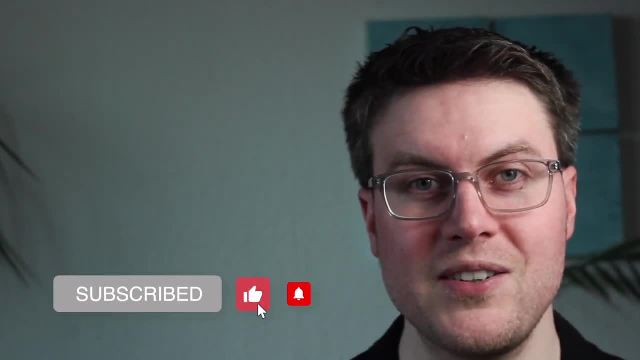 Hey guys, welcome back. We'll continue with the book Python for data analysis. In this video, we're going to cover how we can aggregate and group our data using pandas. This is part of a multi-part series, so feel free to subscribe to the channel to not miss any videos.